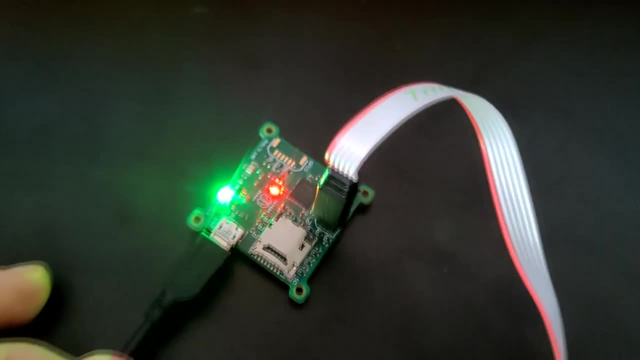 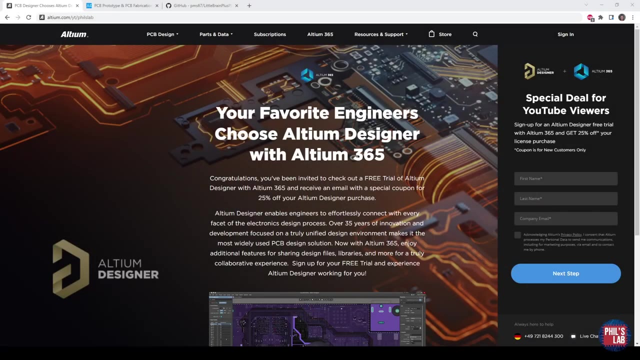 This is the last part of the SensorFusion series of videos, so make sure you've checked out the previous three videos to get familiar with the topic. Thank you very much to Altium for sponsoring this video. The LittleBrain PCB you saw at the beginning was designed using Altium Designer. 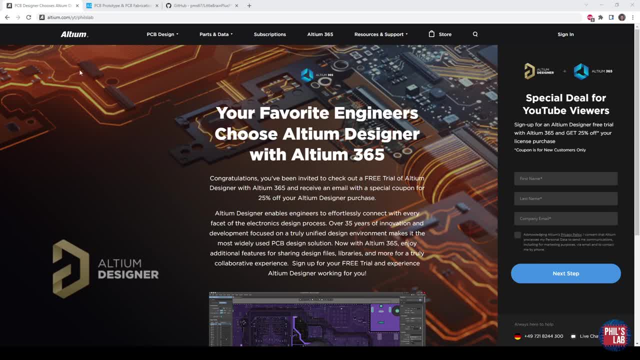 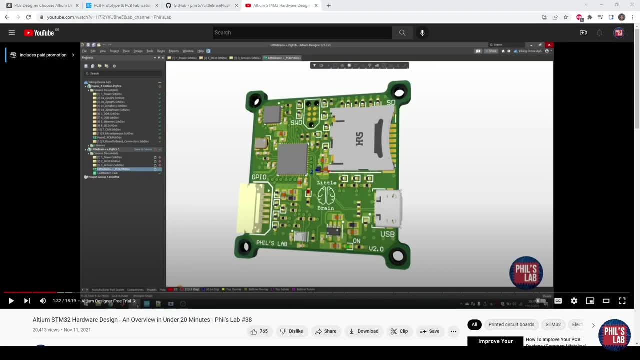 If you'd like to give Altium Designer a try for yourself, you can get a free trial if you go to altiumcom. forward slash yt, forward slash phil's lab. If you're interested in the hardware design aspects of this LittleBrain++ board, I have a video, number 38, giving you an overview of the hardware design in Altium Designer. 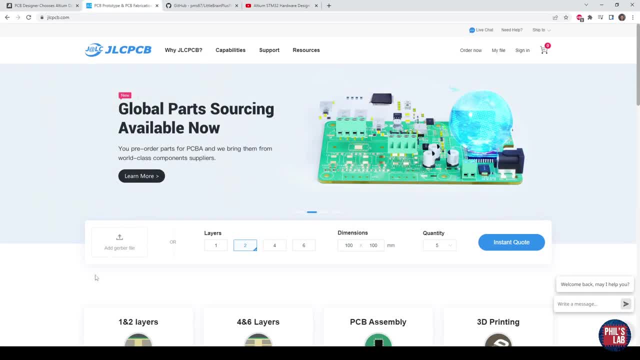 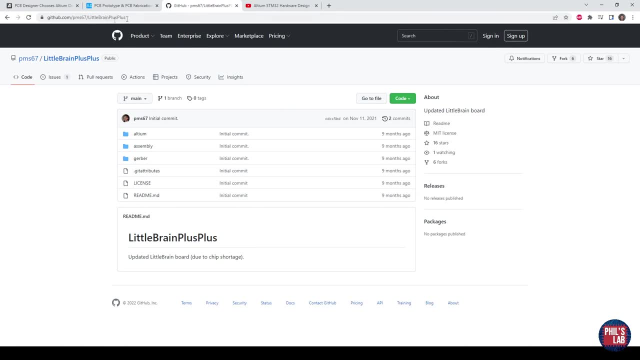 Thank you also to JLCPCB for sponsoring this video. I had the LittleBrain++ manufactured and assembled by them. If you'd like to get yourself a LittleBrain++ board or look at the design files, you can go to my GitHub account at githubcom. forward slash pcb. 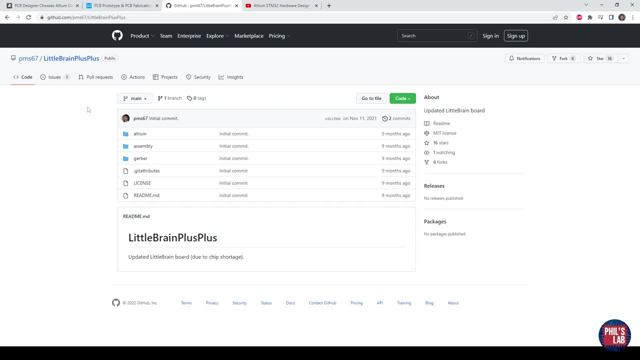 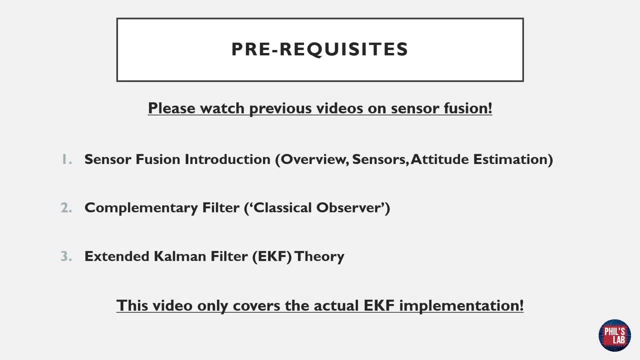 This is the last part of the SensorFusion series and, of course, there'll be some prerequisites that I'll be basing this video on. Please watch the previous videos on SensorFusion. First of all, we have the SensorFusion introduction video On my channel. this is number 33, called accelerometers and gyroscopes. 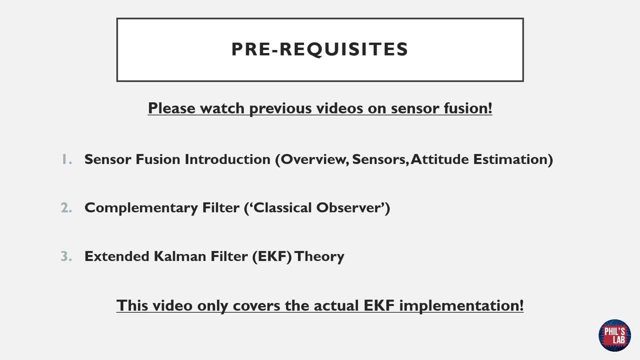 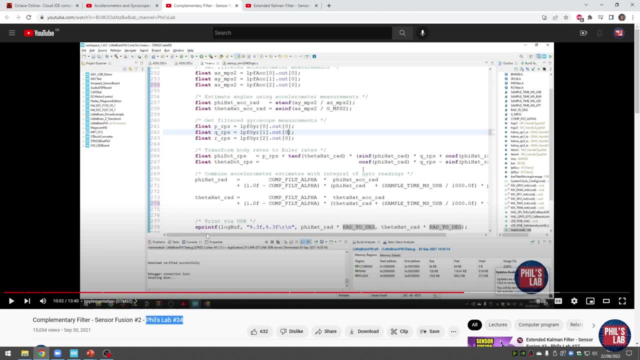 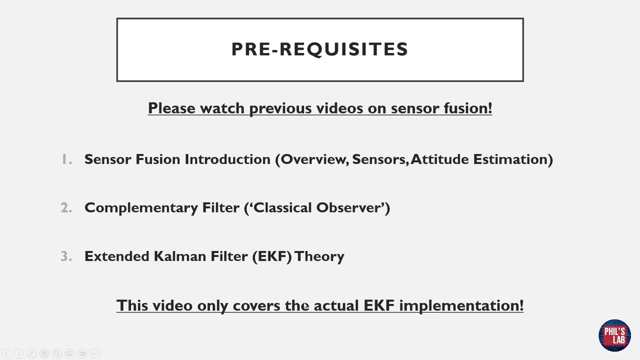 We had a look at the complementary filter, which is one of the most simple types of observers or SensorFusion algorithms, And this is video number 34 on my channel, which also goes into the real-time implementation using STM32 microcontrollers. Lastly, we looked at the Extended Kalman Filter or EKF theory, and a lot of this video will be based on this third video. 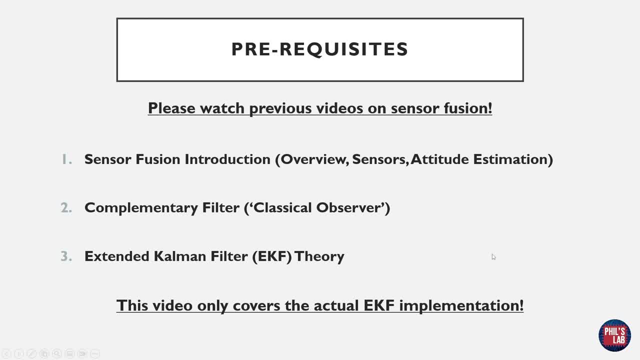 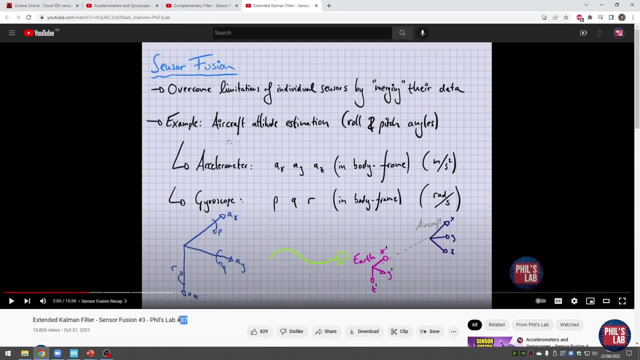 so please make sure to check that out, as I won't be going over the theory in this video. This video then only covers the actual EKF implementation in real-time. The last EKF video was number 37 on my channel. In this video, we first have to look at the low-level firmware before we even get to the EKF part. 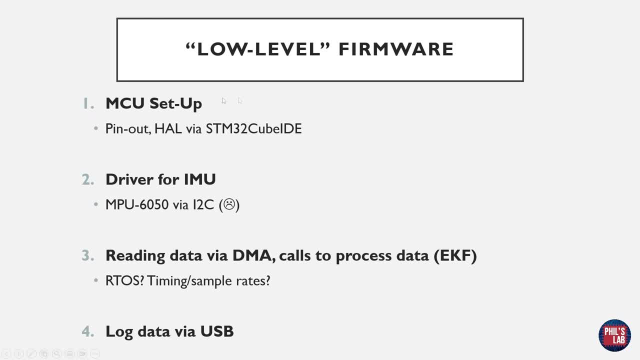 This includes the microcontroller setup, so selecting the pinout, doing the hardware extraction layer via STM32 CUBE IDE. then we need to write a driver for the MPU6050, and I'm using I2C in this example, but I2C really shouldn't be used for any mission-critical or critical systems at all other than really simple configuration. 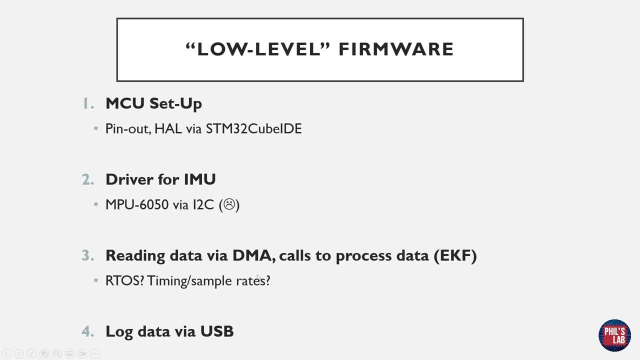 Then we need to read the data via DMA. Once we have this data read and the DMA gives us an interrupt flag, we need to call DMA. Then we call an EKF processing function and you can remember from the last video we have both predict and update functions in our Kalman filter. 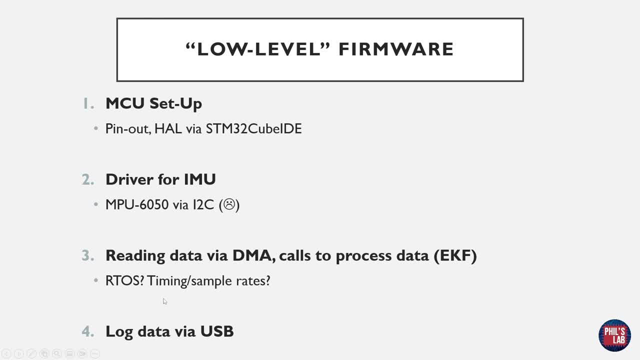 Another option of doing this would be using a real-time operating system, and I've just gone the really simple route, just for demonstration purposes. We also need to ensure accurate timing and fixed sample rates. Lastly, our firmware for demonstration purposes should log data via USB. 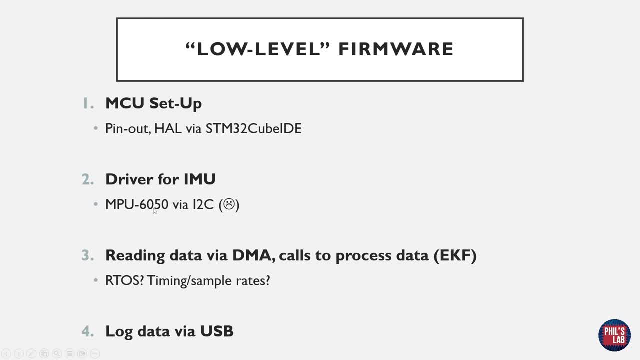 Now I do have several videos on all of these topics, which I'll link to in the description below, so make sure to check those out: how to do proper MTU processing, how to do setup, writing a driver and doing DMA and USB logging. 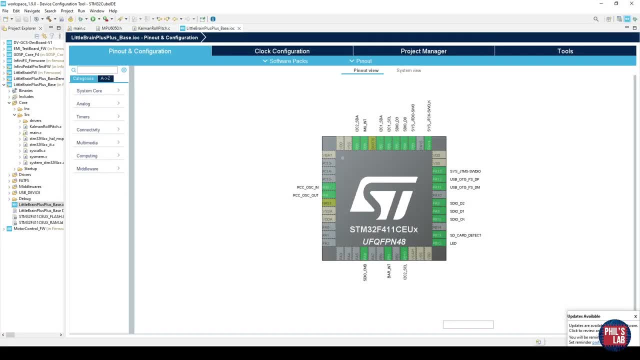 I'll just gloss over the main functions in this video. As you saw at the start of this video, I'm implementing this firmware on the LittleBrain++ board, which contains an STM32F411 microcontroller, and I've really done the pinout for this. 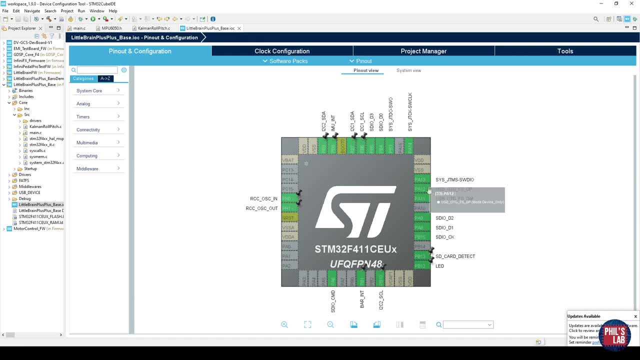 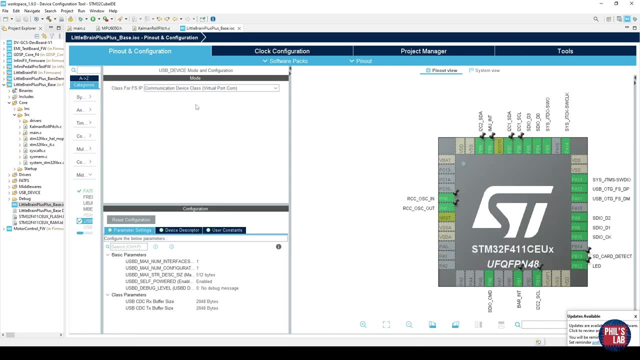 So I've enabled the external crystal oscillator. I've enabled USB full speed I2C, my IMU interrupt and serial wire debug. I have some other peripherals for different sensors, but we won't need this in this video. In middleware I've also enabled the USB device as my communication device class, which is a virtual com pod. 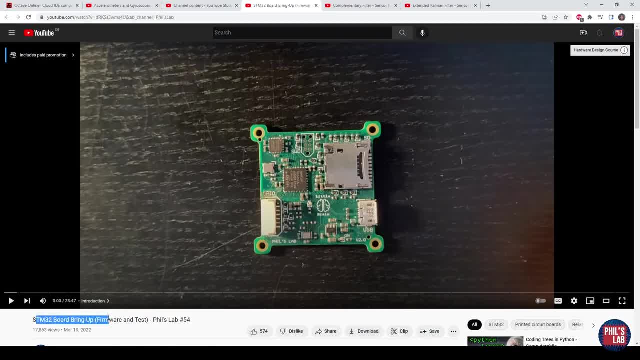 If you're interested in looking at this in more detail, I have a brief video on STM32 board bring-up. that's video number 54, which goes exactly over the bring-up of the basics of this LittleBrain++ board. Of course I have more involved videos on my channel. again, I'll leave the link in the description below. 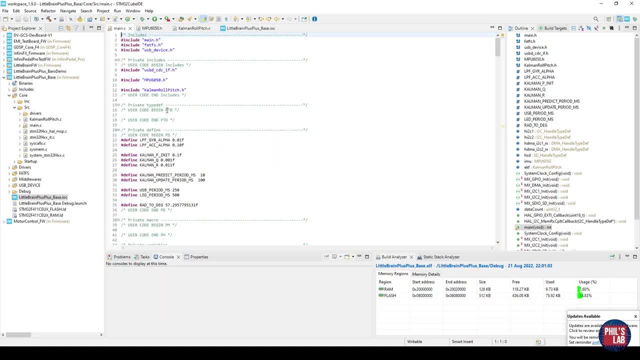 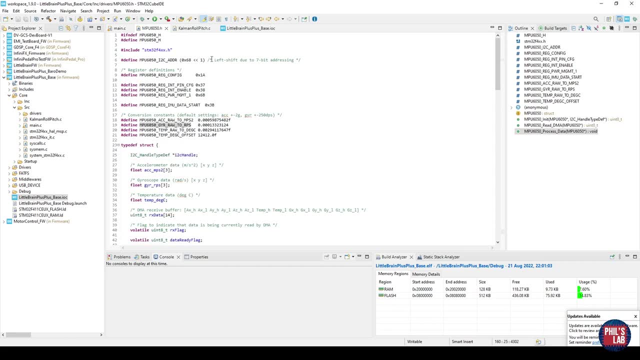 We can briefly look through the mainc code before we move on to the actual EKF implementation, and I'll just briefly show you the IMU driver as well, for completeness sake, The IMU drivers for the MPU6050,. and I've written a really crude driver. I didn't even write a c file. it's all in a container, in a h file. 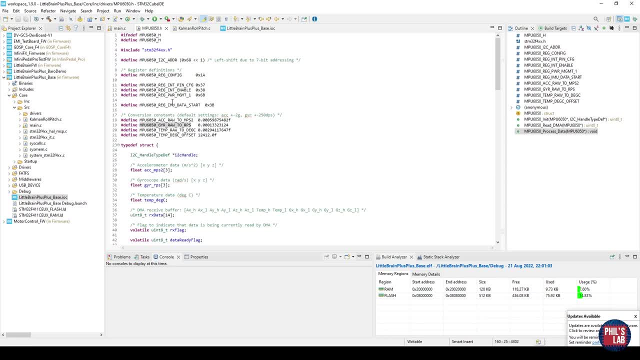 I'm just storing various register addresses which I need to enable the inertial measurement unit to power it up, and then the registers for reading the data. I also have some various conversion factors because I read essentially raw data from the inertial measurement unit. 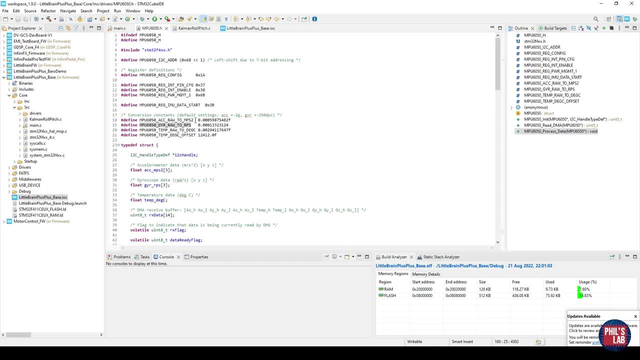 and I want to convert that, for example, the accelerometer data, from raw to meters per second squared. so I have this magic factor over here. I want my raw gyroscope data to map to radians per second. So, RPS, I'm storing all of this data in a struct and then I initialize the sensor to the default parameters. 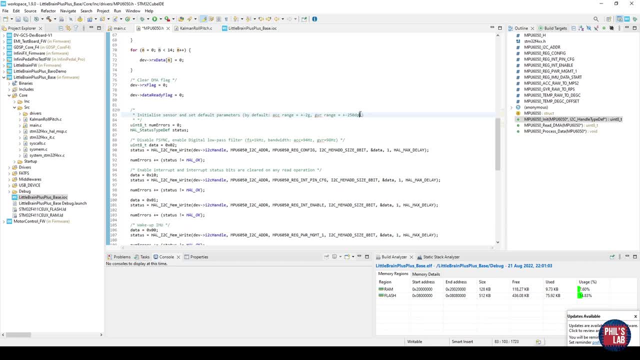 That's, the acceleration range is plus minus 2G and gyroscope range to plus minus 250 degrees per second. Now this, of course, will vary depending on the situation you're in. If you're placing this in a very maneuverable drone, it's very likely that you'll have ranges far higher than these. 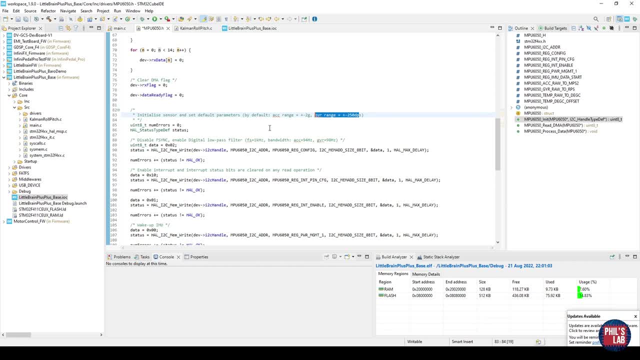 But since I'm just playing around with this on my desktop, the default ranges are perfectly fine. I am also enabling the internal digital low-pass filters, even though we'll be performing some low-pass filtering in software later. So I have a sample rate of 1kHz and I'm limiting my accelerometer bandwidth to 94Hz and gyroscope to 98Hz. 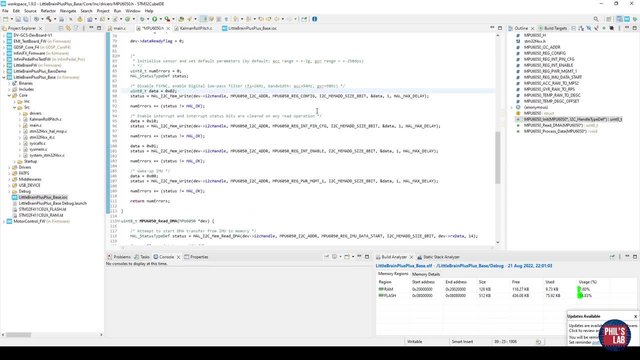 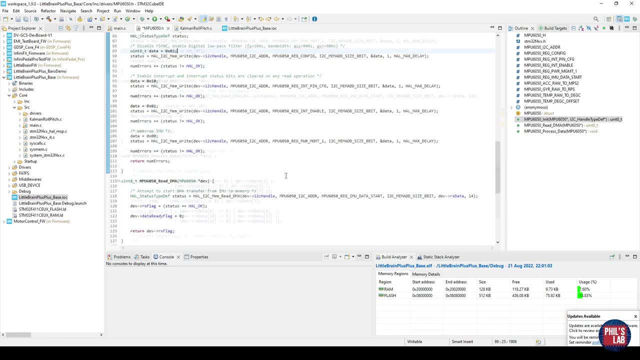 Again, this is situation dependent. Then I'm setting up the interrupt to make sure every time data is ready, my interrupt flag is set and then I can trigger the DMA read And that's all there is to this initialization function. I then have essentially the process or read data functions. 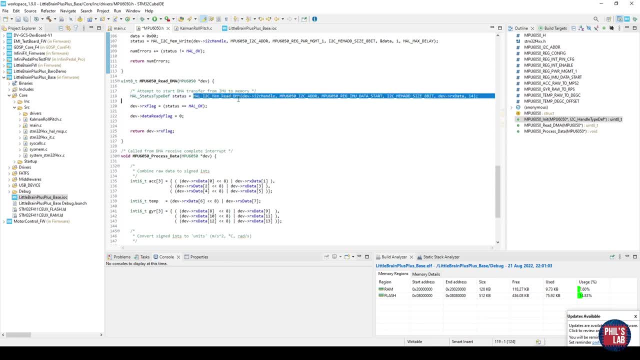 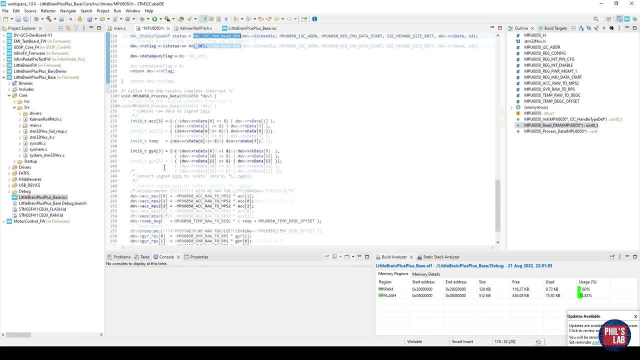 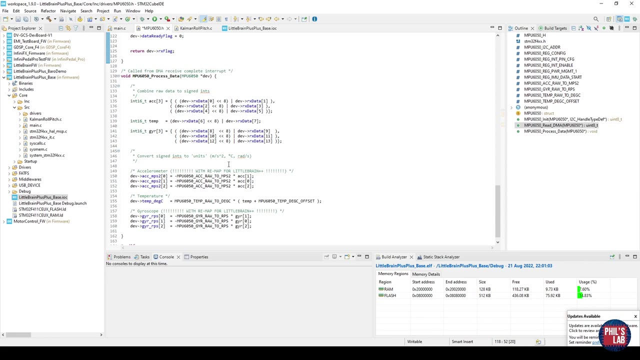 One is the read DMA, which essentially just calls the hardware abstraction layer read DMA and reads all the accelerometer. I also have a small process data function which simply converts from my raw data to my process data, And we'll come back to this because we also have to do an access-free mapping. 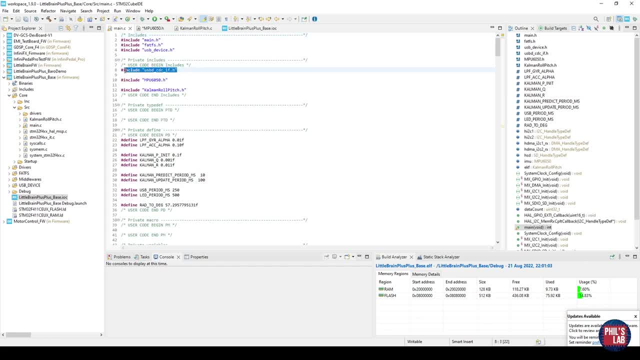 In mainc there's not much special. I'm including my USB drivers, my MPU6050 drivers and then the extended Kalman filter source file which we'll go over later. I have various constants which we'll examine later as well. 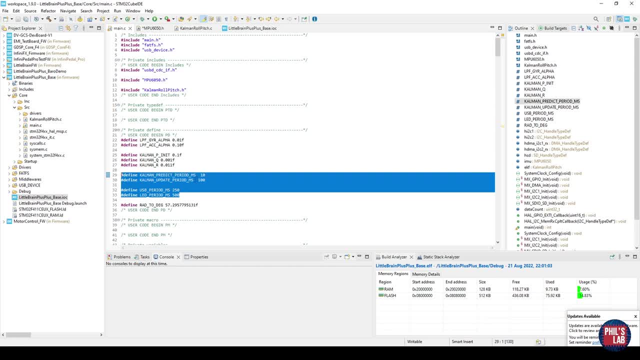 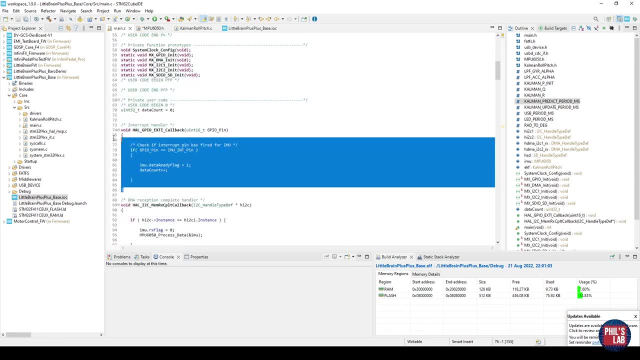 Some things to note are sample times in milliseconds, So I've already set up my predict and update periods, As well as my USB logging period as well. I have an interrupt handler as my callback, So every time, any time the MPU6050 has data ready, it pulls a pin high. 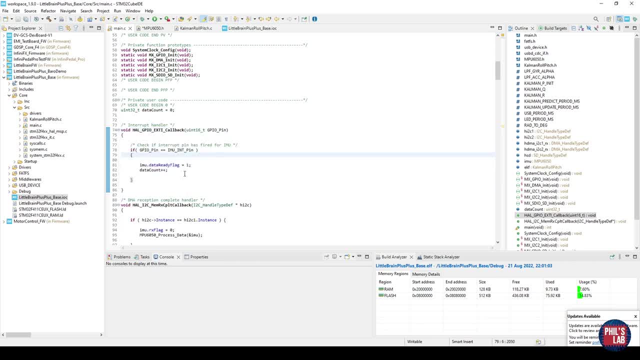 This interrupt handler then says: okay, data is ready, Let's perform a DMA read. Once we've performed the read, essentially I clear the data ready flag and then I process the IMU data In int main. we just have the usual HAL setup. 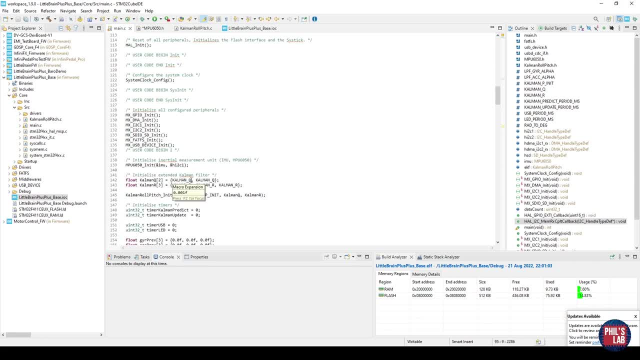 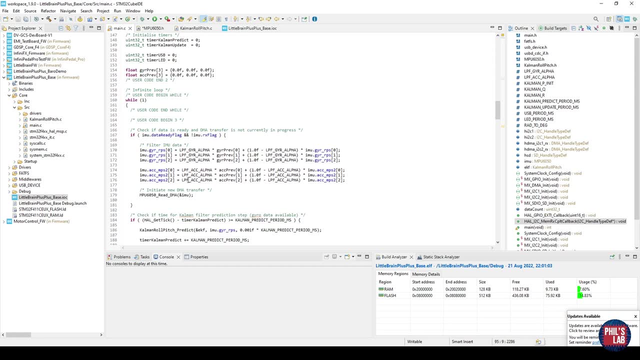 We initialize the MPU6050.. We initialize the Kalman filter- Again, we'll come back to this later- And then we have our main while loop. I haven't used an RTOS and this is a pretty crude implementation, especially timing-wise. 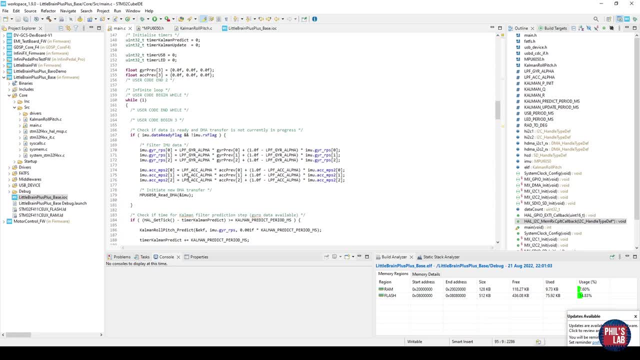 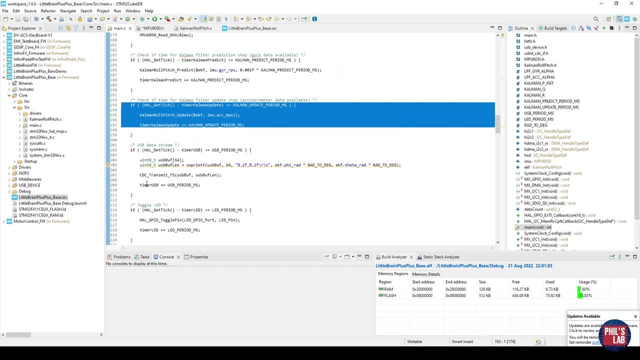 I'm just checking with timers if a certain time has elapsed and then calling functions, For example, filtering my IMU data Or my prediction step of the Kalman filter, My update set of the Kalman filter, Logging and toggling an LED. 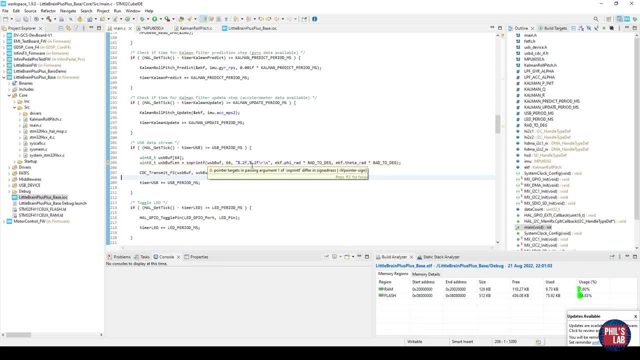 You can see in the logging function, I'm just using the hardware extraction layer or the Virtual Comport device class. I'm simply sending my roll and pitch values, converted from radians to degrees, via USB. So a rather crude, very basic setup. 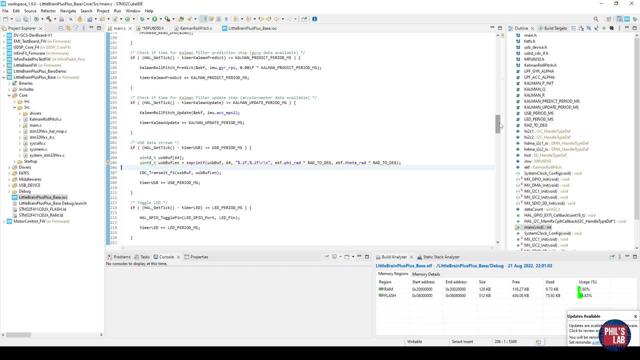 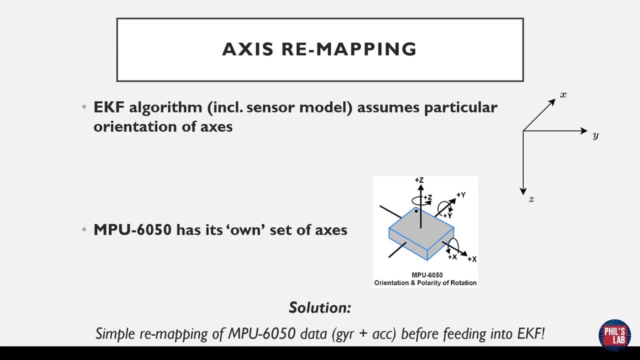 All I'm setting up is DMA streams, sensors and then fixed timing intervals to send data and also to process the EKF data, And that's all there is to this base firmware. As I've hinted at previously, we have to do some things before we go into the actual EKF implementation. 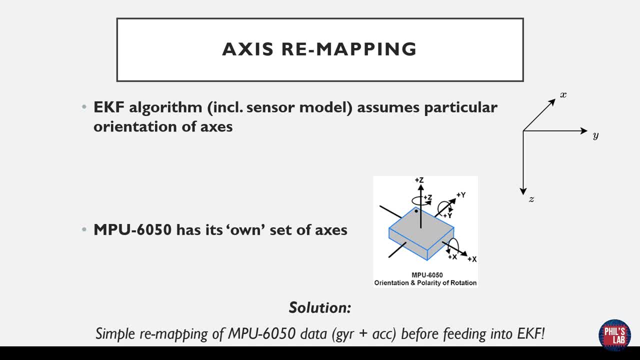 One of these is accessory mapping. If you remember back to our previous videos, our EKF algorithm, including the sensor model we used, for example, for the gyroscopes and accelerometers- assumes a particular orientation of axes, And this happens to be shown on the right. 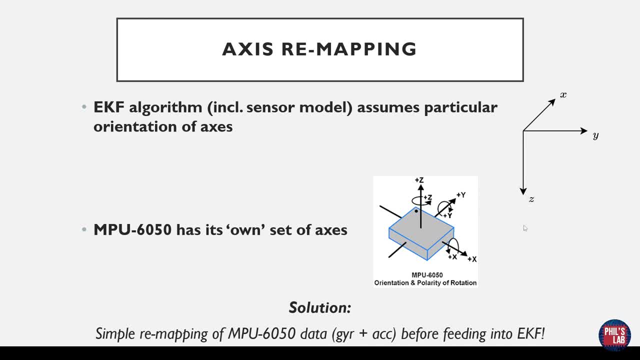 We have X as North, Y as East and Z as Down. However, the initial measurement unit we're using, in particular the MPU6050, has its own set of axes And this is taken from the datasheet shown here, And you can quite clearly see this mapping is completely different. 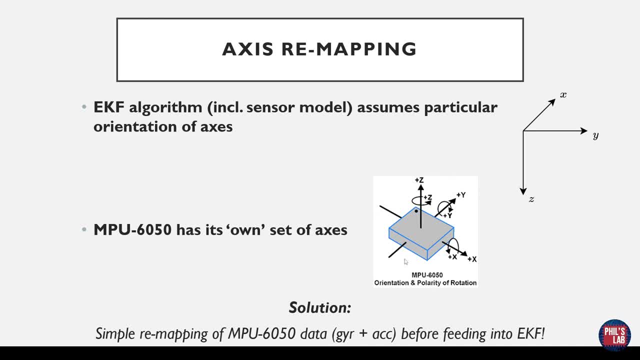 So what we have to do is make sure that the MPU6050 mapping maps to the EKF algorithm's model, Which is assumed. otherwise we're going to get completely rubbish data out. This is actually fairly straightforward. Now, there's better ways of doing this. 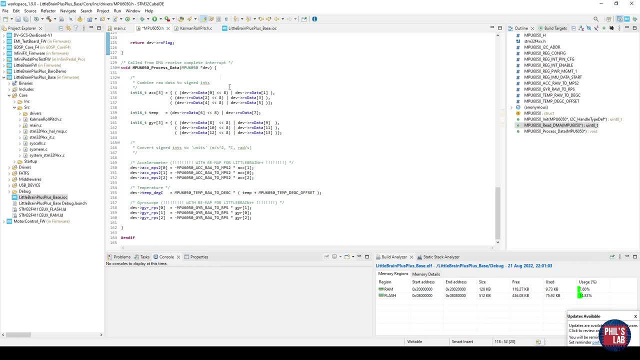 Rather than just doing this in the MPU6050 driver, of course, Because this driver might be used in a completely different project, But since I have this pretty much just local to my EKF, I've just put it in here. Anytime I set my STRACTS accelerometer values, I take my raw data and then remap it. 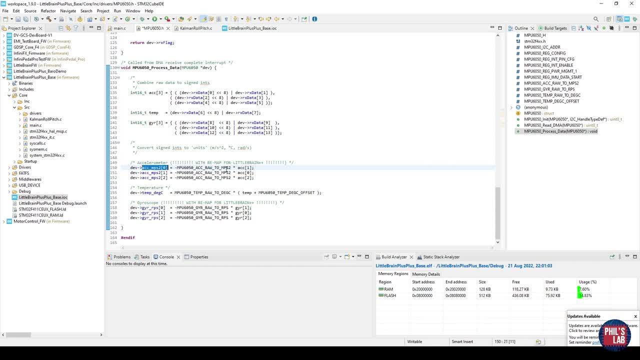 For example, changing the sign and also saying the X axis is actually the MPU6050's Y axis, Or the EKF Y axis is actually the MPU6050 X axis, and so forth. I need to do that both for the accelerometer as well as for the gyroscope. 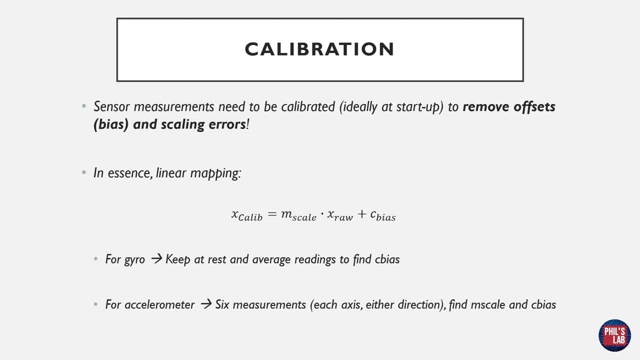 Calibration is a huge topic in its own right. I'm just going to briefly gloss over it with this slide, But keep in mind this is one of the most crucial factors for having a successful sensor fusion implementation. Raw sensor measurements are typically biased or distorted in some way. 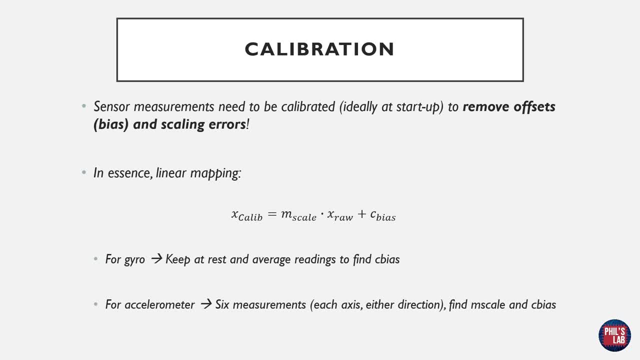 So the sensor measurements need to be calibrated. Ideally, this should be performed every startup, or at least periodically. This is to remove offsets, which are typically known as biases and scaling errors. In essence, we have a linear mapping. we will perform in the most simple case. 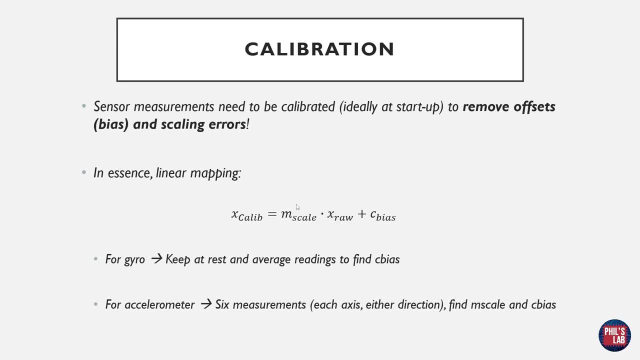 We have our raw sensor data. We have to adjust it with a scale and add a constant or bias to it to get our calibrated measurement value, which we then feed into our remaining algorithms. In essence, for gyroscopes, the easiest way we can do this is keep the gyroscopes at rest. 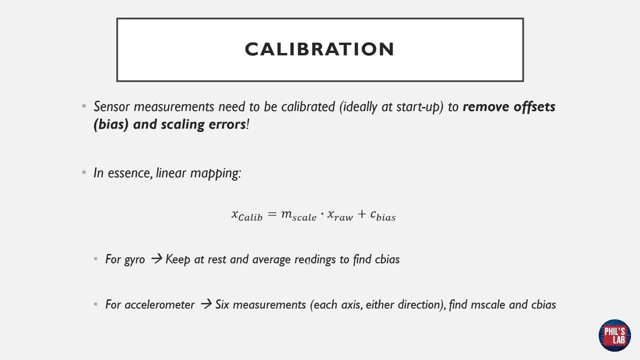 average the readings. so add up all of the readings, divide by the number of readings you have and find C bias or the offset for every axis. Then later on we can subtract C bias from every measurement to have our calibrated measurements For accelerometers. that's a bit more complicated. 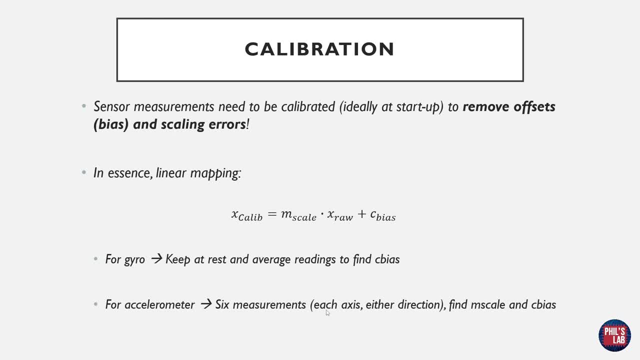 We need six measurements at least, so each axis aligned in either direction- positive and negative- And this allows us then to find the scale factor and the bias value. Of course, you can imagine, keeping these devices at rest will be hard with external influencers. 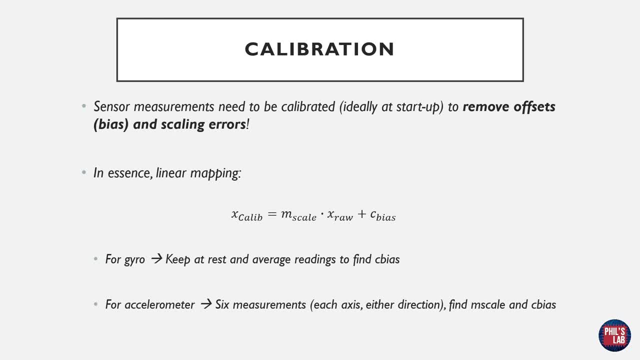 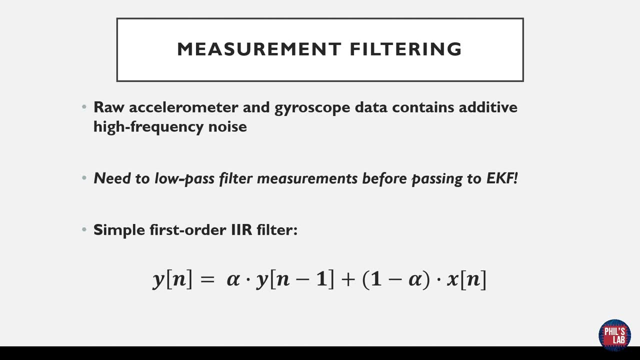 as well as aligning these axes properly to give us plus minus G in either direction. So calibration is a huge topic and typically requires specialized equipment to perform properly. Another aspect is that we saw in previous videos raw accelerometer and gyroscope readings after they've converted from the very raw values. 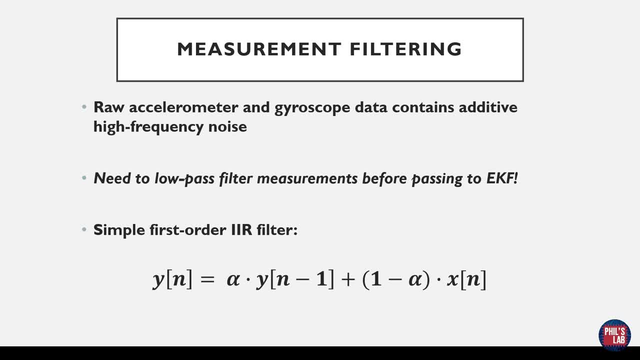 from the MPU 6050 to meters per second squared and radians per second. these will contain additive high frequency noise, And this is pretty much unavoidable. So you could get higher quality sensors, which will in turn, be more expensive. You can use a lower bandwidth digital filter, for example, directly in the IC. 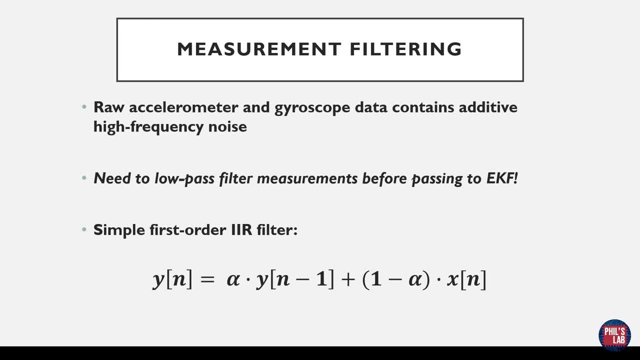 And we're essentially doing the same thing. It always pays off to do some additional measurement processing in terms of low pass filtering, And this applies both to the accelerometer as well as the gyroscope. We use a low pass filter the measurements before passing these to the EKF. 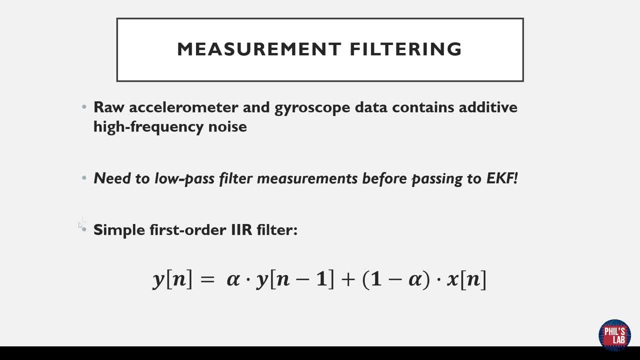 From previous videos you will know. any reasonable and fast filter is a simple first order IRR filter, Digital filter employing feedback. I have an extended video on IRR filter design on my channel. Again, I'll leave a link to this in the description below. 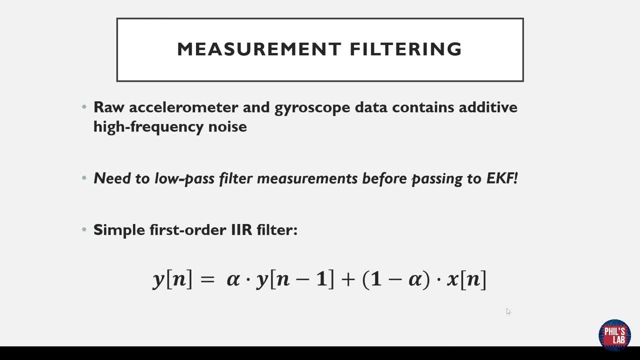 An essence filter we're using before passing these measurements to the extended Kalman filter is this simple discrete time difference equation at the bottom here Our output is Y at sample N And our input is X of N. So X of N would be our raw accelerometer and raw gyroscope data. 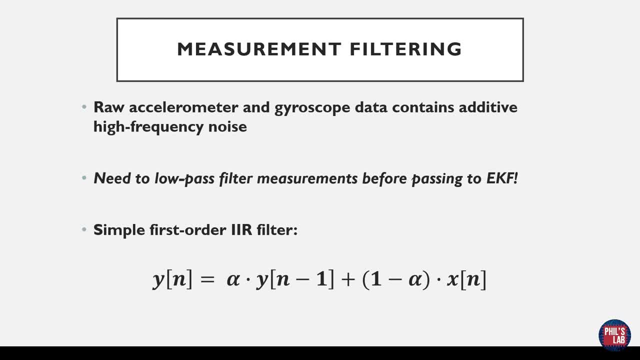 And of course we need three channels of accelerometer and three channels of gyroscope. So we'll have six instances of this filter. Alpha is our filtering coefficient, which goes anywhere from zero to one. If we have alpha equals zero, we essentially we have no filtering. and Y of N is X of N. 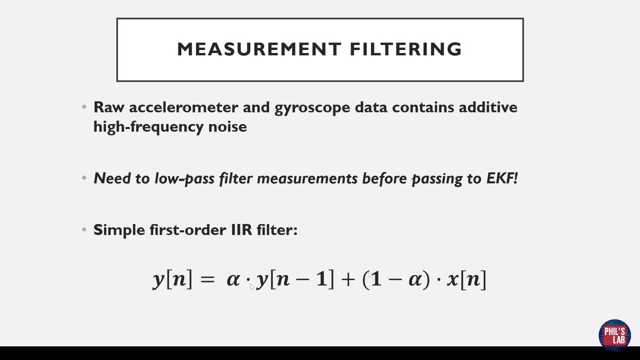 So the output is the input of the filter. As alpha goes towards one, we take more of the previous output of the filter into account rather than accepting the input. So as alpha goes to one, we perform more and more filtering, As is usual with sensor fusion. there is no direct way of determining alpha. 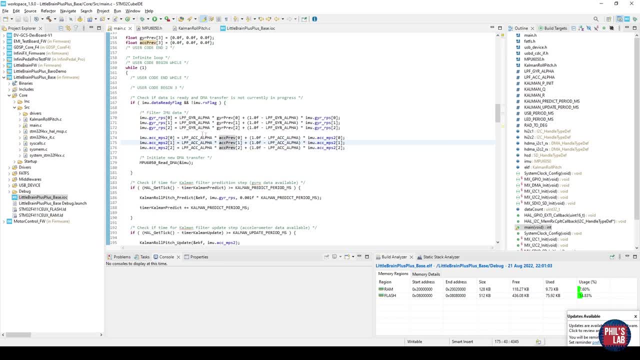 And this is something we have to play around with and also tune In a software implementation. in my main while loop, I'm checking if the IMU data ready flag has been set and the DMA transfer is not currently in progress. If that's the case, I can filter my IMU data. 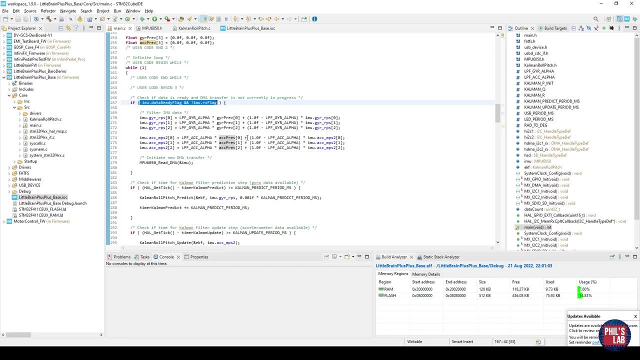 Remember we have to do this for all of the gyroscope data and all the accelerometer data. I have defined a low pass filter gyroscope alpha. You typically want to keep these separate. Gyroscope data contains a lot of high frequency information, So you don't want to filter that as heavily as, for example, the accelerometer data. 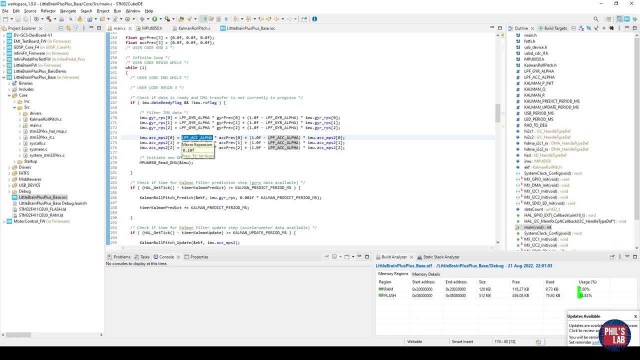 And that's why the gyroscope alpha is 0.01 in this case, And the accelerometer alpha is 10 times higher at 0.1.. Of course, you'd have to play with these values. All I'm doing is then implementing the difference equation. 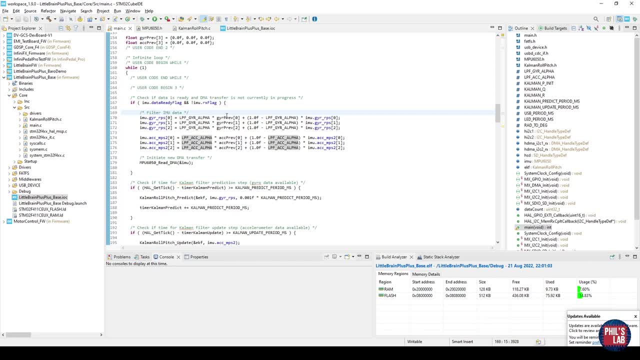 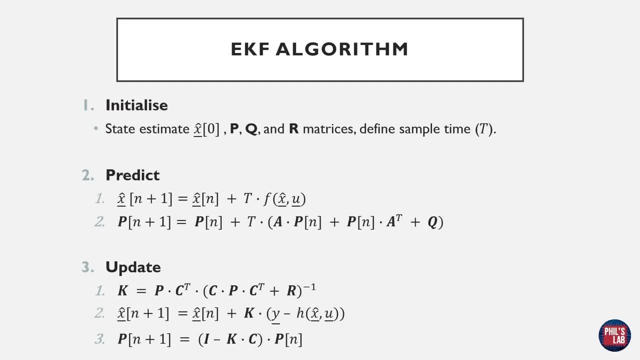 So the current filtered gyroscope data is the previous gyroscope data times, the alpha plus one minus the alpha times, the current gyroscope data. Same thing for the accelerometer. We're pretty much ready now to look at the EKF algorithm and in particular the implementation. 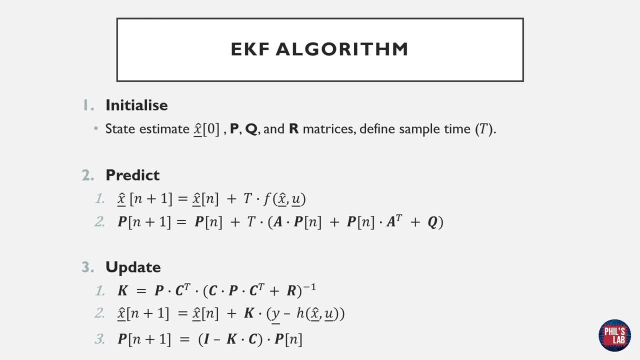 Let's remind ourselves of the algorithm. There are essentially three steps, two of them repeated. The first is to initialize the EKF. So we have a state estimate. In our case we're trying to estimate roll and pitch angles, So our state estimate is X hat at sample time zero. 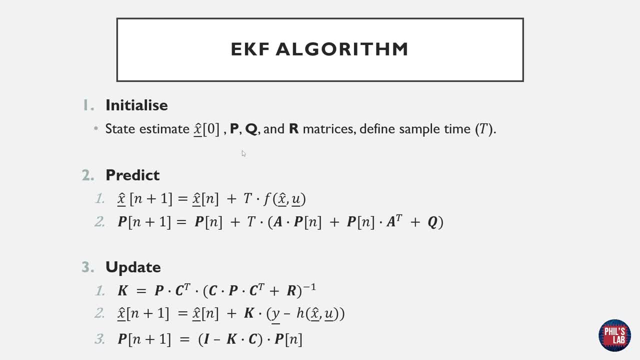 And of course X hat is a vector because it's roll and pitch. P, Q and R are matrices. So P is our essentially error covariance of the current state. So how uncertain the algorithm thinks our state estimate is. Q and R are noise and error matrices. 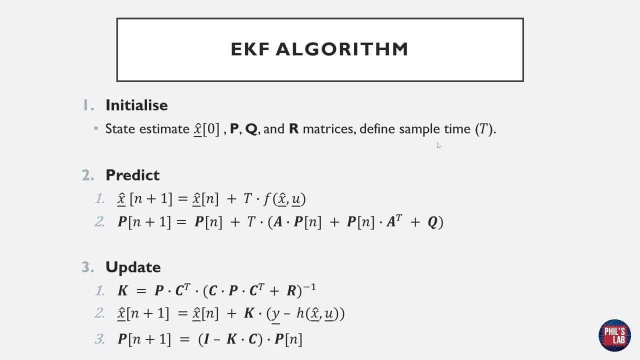 Q for the process and R for the measurements. We also need to define a sample time. So what time is there between prediction steps and what time is there between update steps? Predict and update oftentimes can come together, but usually they are separate. 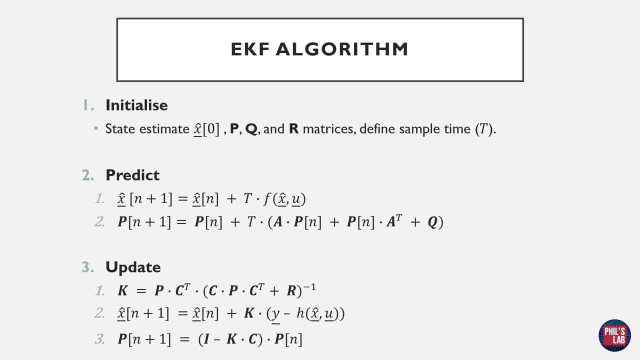 For our prediction step. we'll have sensors that update frequently, for example the gyroscopes, And our update step. we might have sensors that update slowly. This could be GPS units, lidars and so on. Our prediction step will be concerning the gyroscopes. 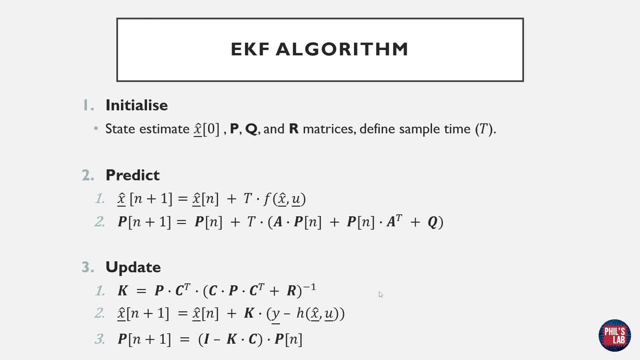 And our update step will be concerning the accelerometers, The prediction step. we have our state transition function F of X and U, which is essentially the rate of change of our model of the state estimate. So it's X dot. We can perform simple Euler integration. 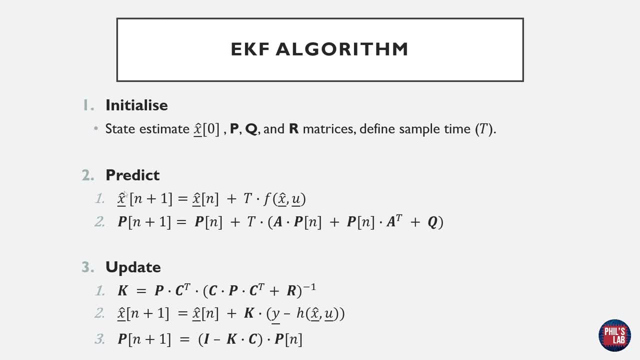 X dot times. T plus the previous state gives us our new state, And that's our prediction step. Again, all of this was covered in the previous video. We then also have to update our error covariance matrix using this formula below here, And we'll see exactly how to implement that numerically: 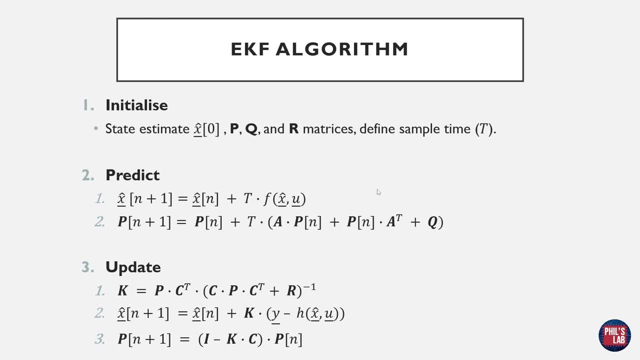 or how we get an actual expression that we can implement in a programming language in just a second. Our update step is different. We have to compute the Kalman gain And this unfortunately involves a matrix inversion. Luckily for us, we will only have to invert a 3 by 3 matrix. 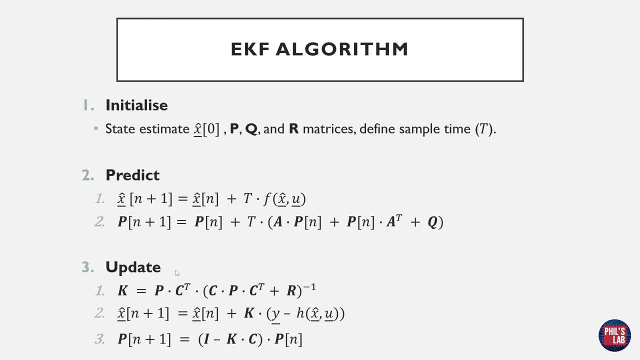 But you can imagine how expensive this operation is for larger system dimensions. Then we apply the correction step, which is essentially the Kalman gain, depending on our accelerometer measurements, And this depends on the Kalman gain as well, And we can also update our error covariance matrix. 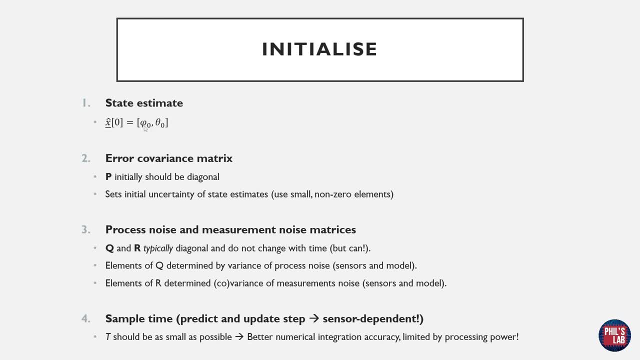 Let's look at the initialize step. first. To initialize, we initialize our state estimate And this will contain the roll at time 0 and the pitch at time 0.. And for most cases, we will just set these to be 0.. 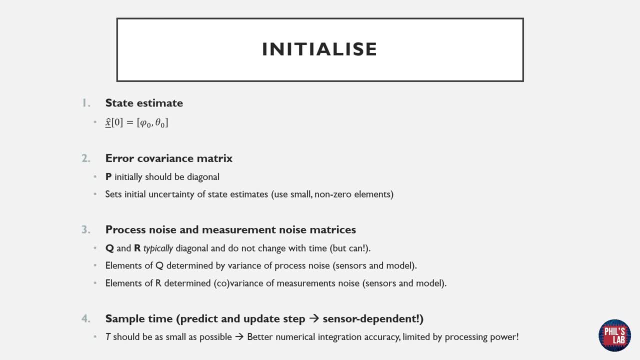 I have my board like flat on my table and I'm assuming that's a roll and pitch of 0.. Of course, the table could be misaligned, the sensors misaligned, and so on. This is our initial state estimate, So really easy to set up. 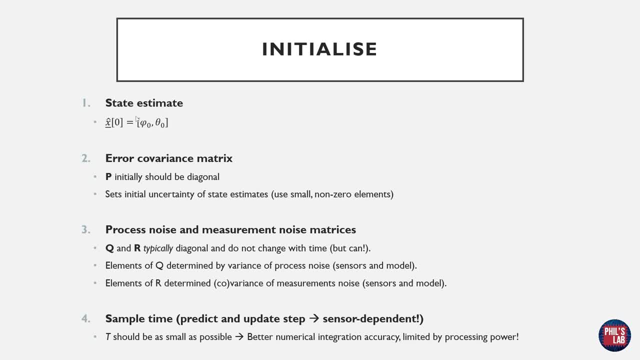 We could, of course, use the accelerometer to give us initial state estimate, giving a very crude estimate of inclination and roll. Then we have the error covariance matrix, And it's starting to become a bit more complicated. P, our error covariance matrix, gives us an estimate of how uncertain our estimates are. 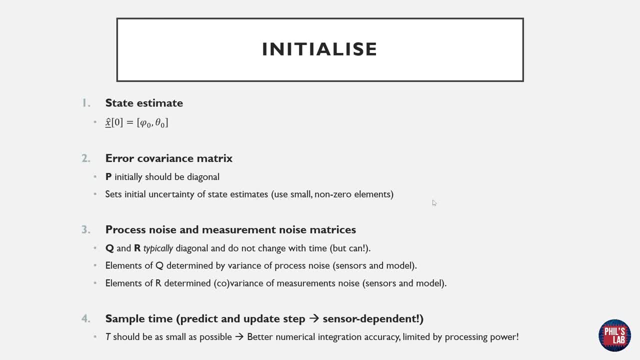 Initially, P should be diagonal and typically small, non-zero elements, And the order of magnitude might be something like 0.1, 0.01, that kind of order of magnitude. It's hard to generalize. We also have our process, noise and measurement noise matrices. 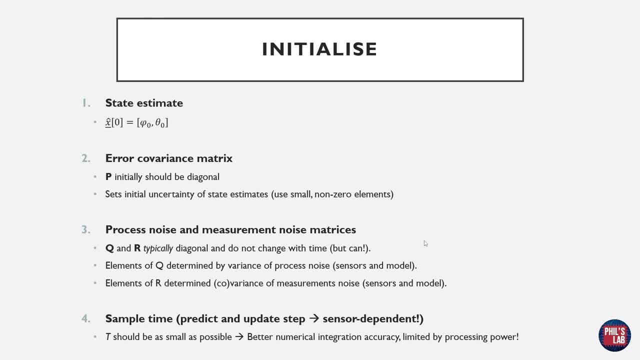 These are Q and R respectively And typically these will be diagonal And in our case we will not change them with time, But it's very sensible Sometimes to make these time varying. The elements of Q, the diagonal elements, can be determined by the variance of the process: noise. 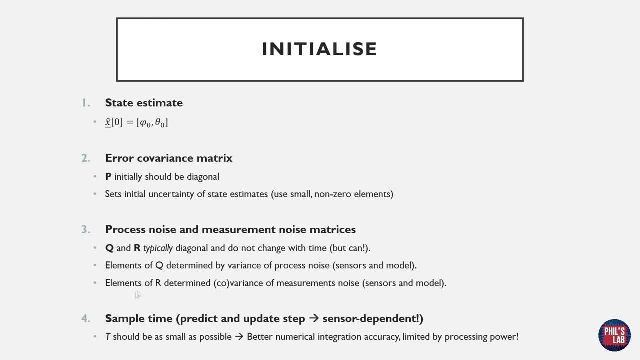 So that takes into account our sensors in the model, And the elements of R are determined by the covariance of measurement noise. Including the sensors and model. again, Now, this is a very high level description of how to determine Q and R And oftentimes, in practice, and even though you might be able to get them directly from the model and sensor data sheets, 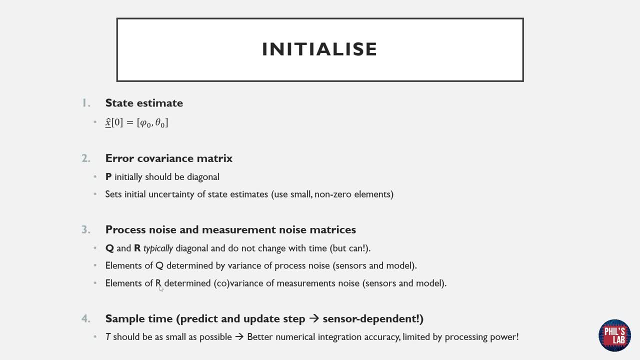 in practice you will have to do quite a lot of tuning of Q and R to make sure your EKF performs appropriately. If Q and R aren't set properly, your state estimates will diverge, It will be an unstable filter, and so on. 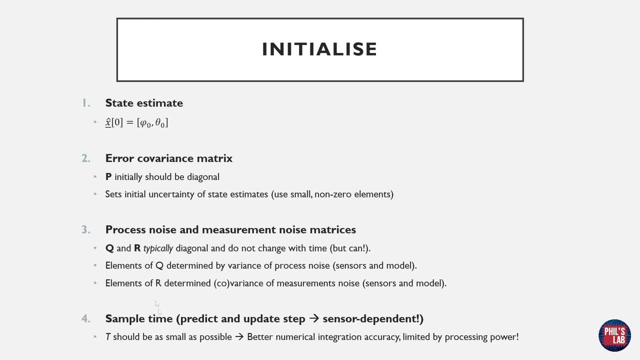 So it pays off to spend some time tuning Q and R. Lastly, of course, we also have the sample time. Predict and update steps will be sensor dependent. It depends on when we get our rate updates from the gyroscopes or when we get our accelerometer measurements. 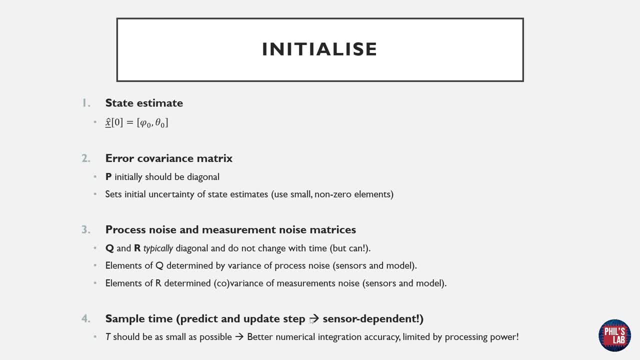 And these might be different sample times. In any case, the sample time should be as small as possible, Especially for the prediction step. We get better numerical integration accuracy With such a simple oil integration method. This, of course, is limited by the processing power. 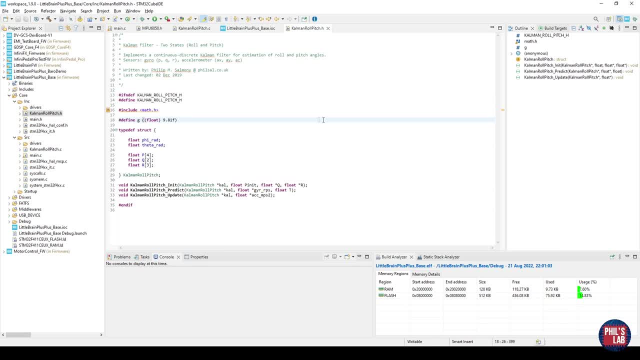 Now, for the first time, let's look at the actual code of the Kalmanfeld implementation. This is incredibly crude, very simple and simply for demonstration purposes. Again, this shouldn't be used in any sort of critical system. This is the header file and we have three functions. 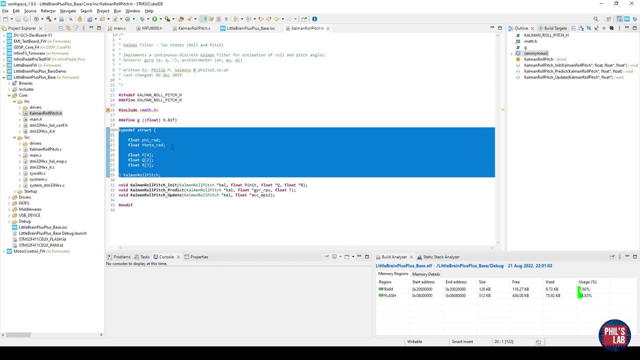 Initialize, predict and update, As well as the struct. The Kalmanfeld of struct takes our state estimates, Phi in radians and theta in radians, That's roll and pitch respectively. It takes our error covariance matrix, Which is a 4x4 matrix. 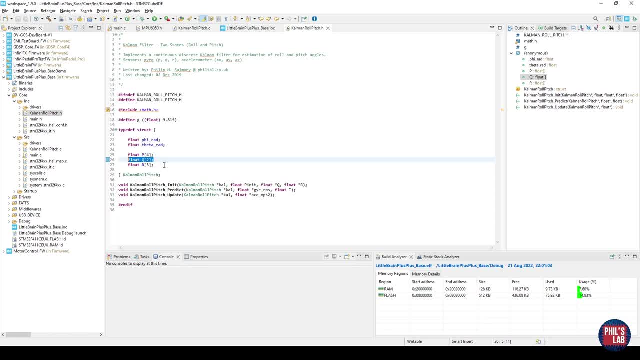 Our process, noise matrix Q, Which is a 2x2 matrix, And our measurement noise matrix, which is a 3x3 matrix R. The initialization function then takes the struct One initial value for the error covariance, And this will place this value along the diagonal. 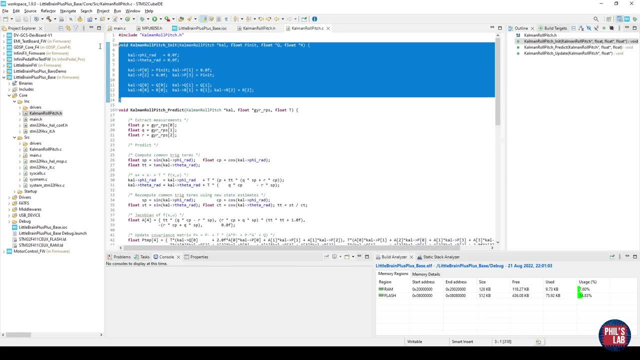 And then pointers to Q and R matrices. In the actual function itself we can see we're initializing the state estimates to 0. Just by default, Filling in the diagonals of P And filling in Q and R. You can see I've set Q and R to just be vectors. 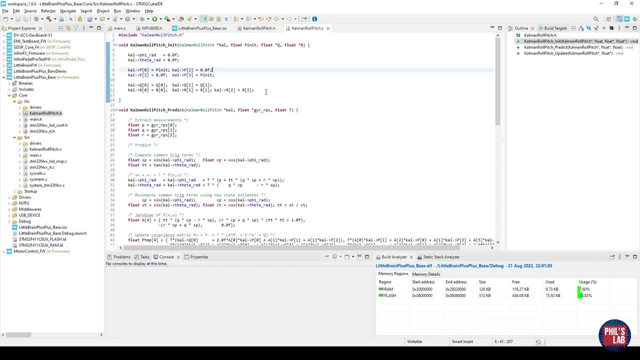 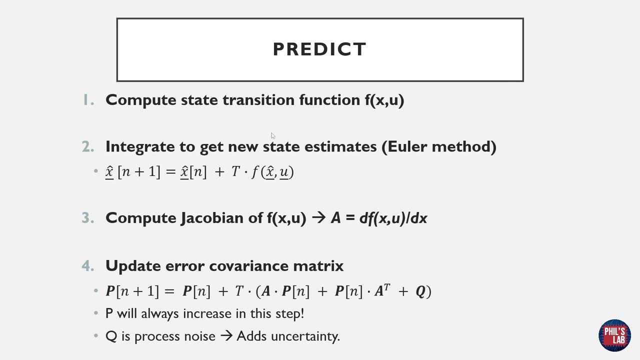 Because I'm assuming these are diagonal matrices, So the off-diagonal elements will always be 0. Is my assumption. Then we have the prediction step, And this is simply taken from the previous video. We have to compute our state transition function. 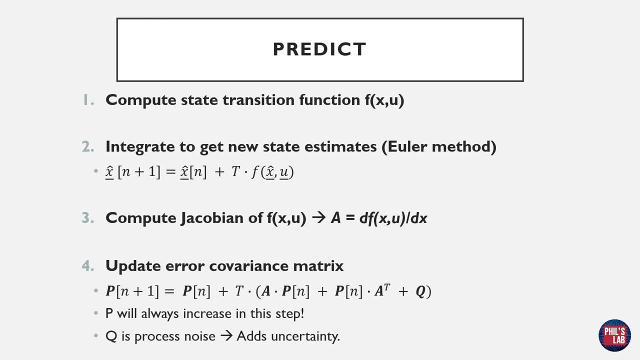 Which is essentially x dot. So how does our state change with respect to time? We use that state transition function and integrate it, In this case using the Euler method. Then we need to compute the Jacobian of F, Which is essentially df, by dx. 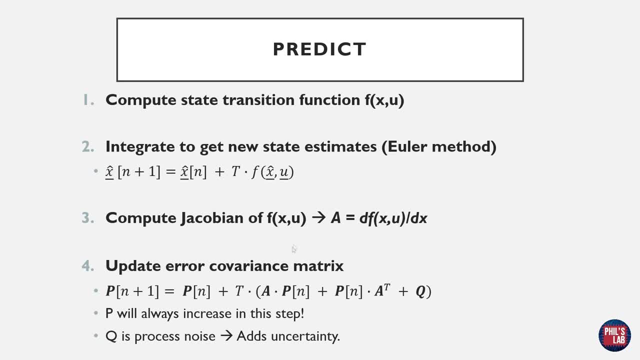 Which will give us a matrix A And we use that matrix A With our previous error covariance matrix And our process noise Q To update the error covariance matrix. In our prediction, step P will always increase, Q is process noise and that will add uncertainty. 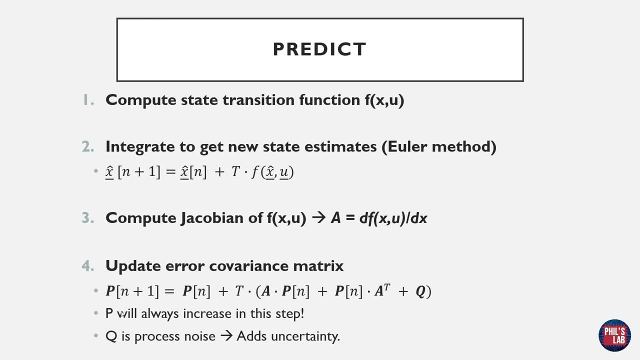 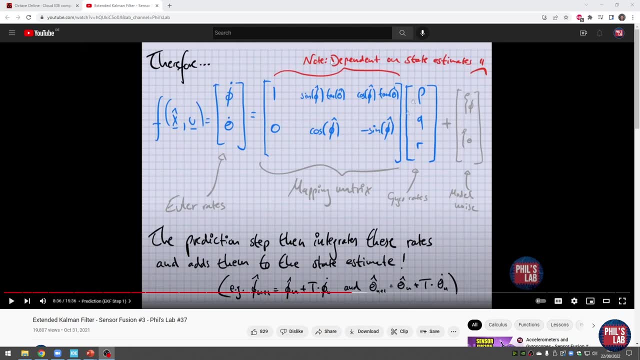 Our uncertainty in our measurement will go up, Which is reflected by the magnitude of P increasing. If you look back at the last sensor fusion video, number 3.. We can see this is our state transition function. We have some sort of mapping matrix. 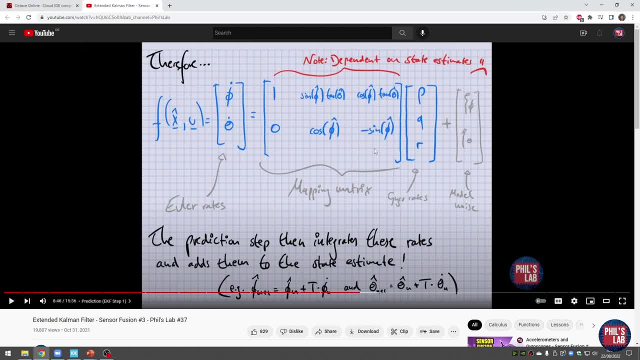 And the gyro rates And some sort of model noise. So all we have to do Is multiply our gyro rates, Which we get from the filtered measurements of the sensor, Multiply it by this matrix And this is our state transition function. If we go to the prediction function, 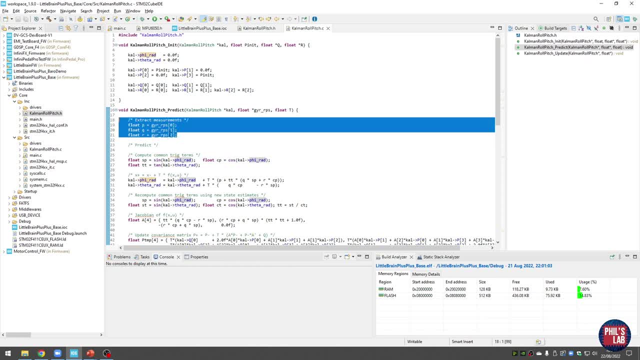 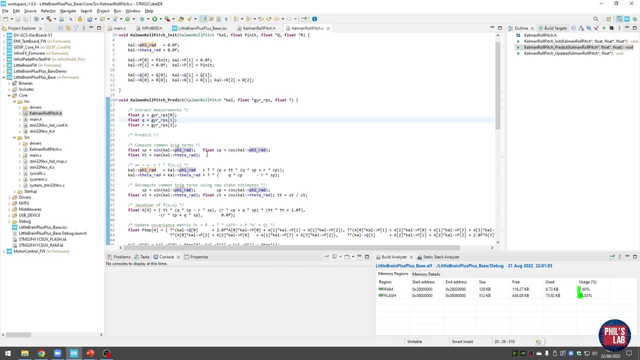 In STM32Q by DE. I am extracting the measurements, So P, Q and R, Which are my gyro radian per second measurements, And X, Y and Z axes. Then I am starting my prediction step. What I like to do is compute common trig terms. 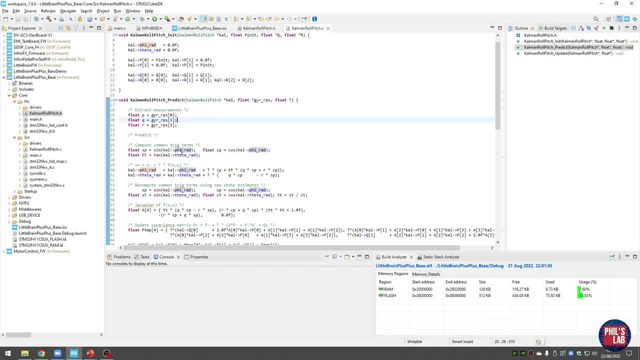 This not only cleans up the code, But often times, for example, the sine of the roll angle I have to use more than once. So I pre compute the common trigonometric terms, Then I perform my Euler integration, My new roll angle phi. 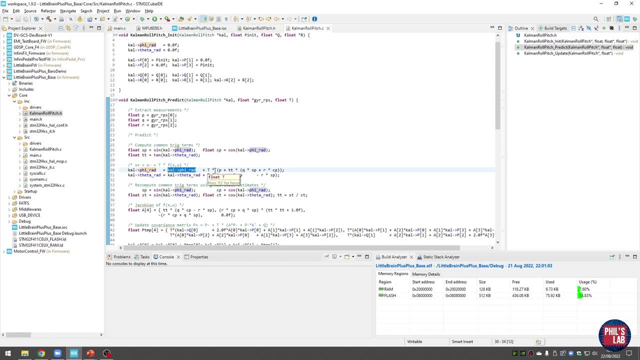 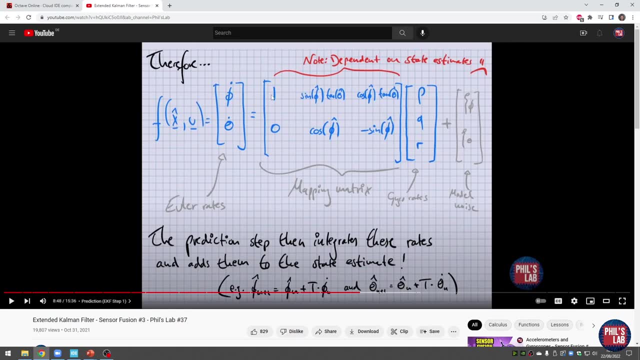 Is my old angle: phi Plus T times the state transition function, And that is simply This: matrix times the gyro rate, And this will then be the first row. So it's P plus Q Times sine phi tan theta, Plus R times cos phi tan theta. 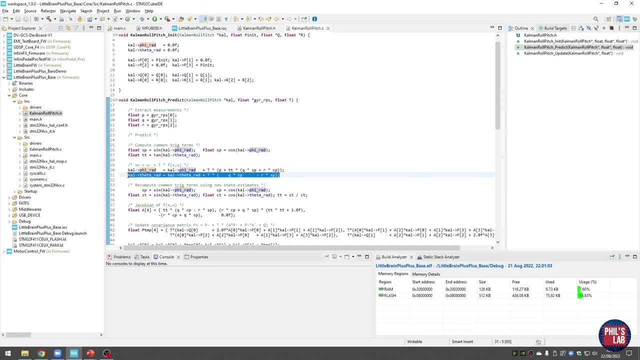 And that's all I have done here. Similar for theta, which is my pitch angle. I do exactly the same thing. Now I pretty much have Two predictions of my roll and pitch angles. I have to re-compute my common trig terms. 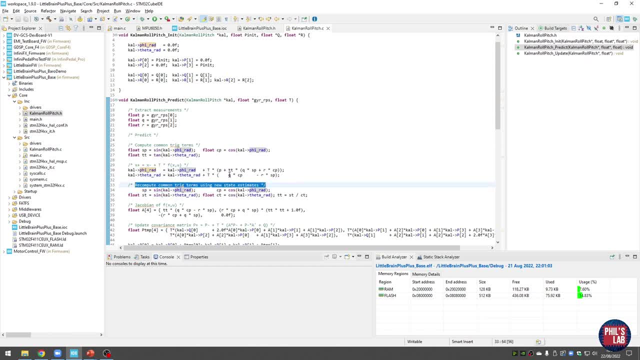 Using these new state estimates Because these are different To the trig terms we computed earlier. So I am re-computing my common trigonometric terms Using the new state estimates. Once I have that, I need to compute the Jacobian. 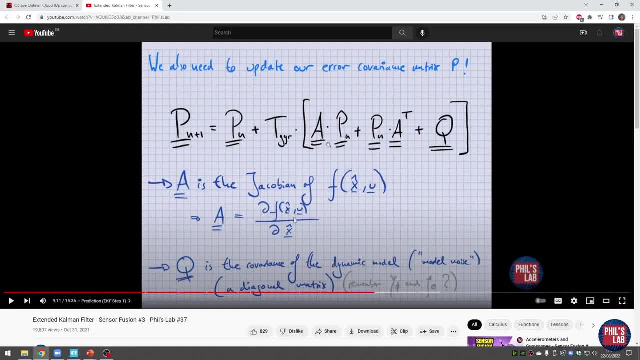 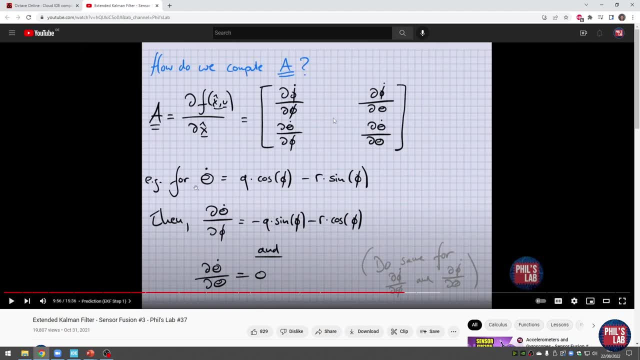 Of my state transition function And remember the Jacobian is Partial DF of XU by DX. The question is, how do we do that Without making any errors? I could, of course, do this with pen and paper, Especially for larger matrices. 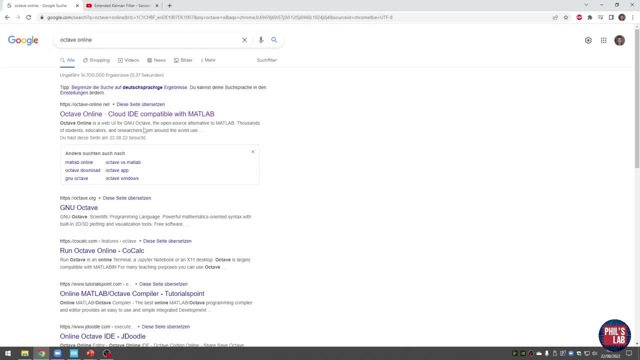 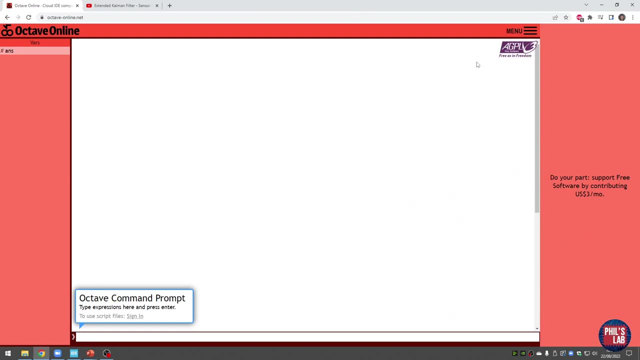 I'll show you how to do this using the MATLAB symbolic functions. There's a free version of MATLAB Called Octave And there's even an online interpreter At octave-onlinenet, And we'll use that because this is accessible to anyone. 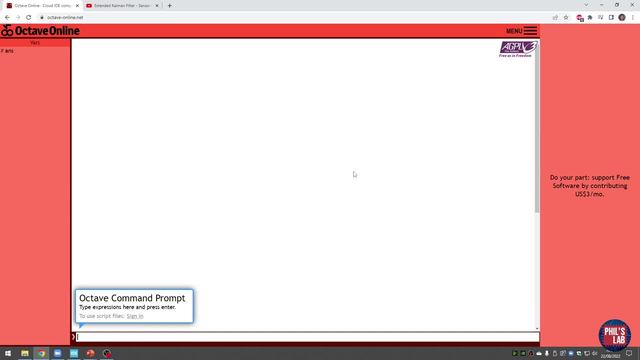 We need to create some symbolic variables And let MATLAB- or Octave in this case- Do the work for us. So I'll create symbolic variables P, Q and R, Which will then load the package, And I'll also create symbolic variables for roll and pitch. 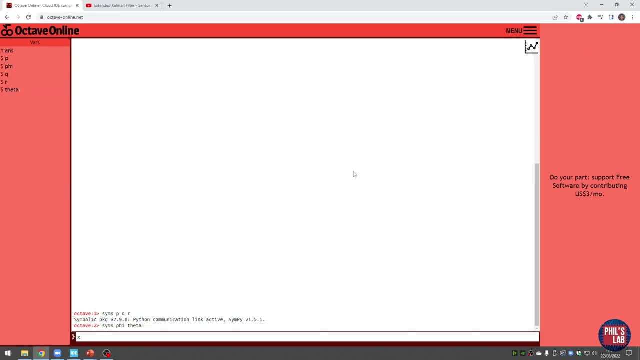 Which I'll call phi and theta, And then I'll create my state vector X and I'll make that a column vector With phi and theta. If I type in my state transition function F, which we got from the slides, You can see I have this vector as well. 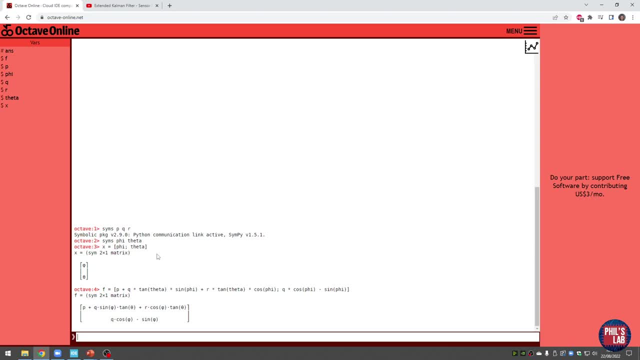 The question is, how do we get the Jacobian from this? And luckily MATLAB and Octave have a very handy function, So I can say: A, which is my Jacobian, Is simply Jacobian of F. With respect to my vector X, It has now computed my Jacobian. 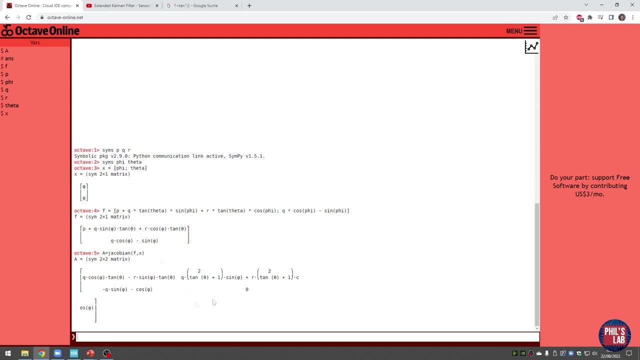 You can see, it hasn't simplified things Too much And we can do some minor improvements. For example, 1 plus tan squared theta, That means this is sec squared theta, Or 1 over cos squared theta. So, taken just simply from these identities, 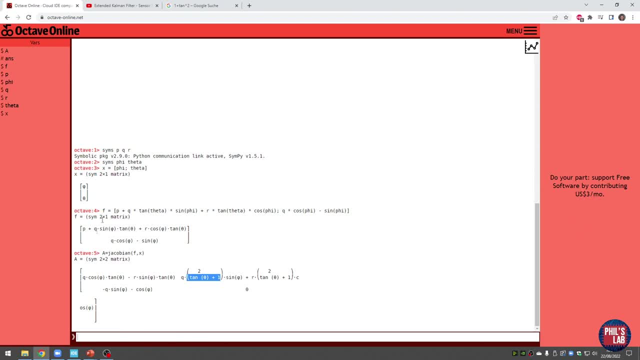 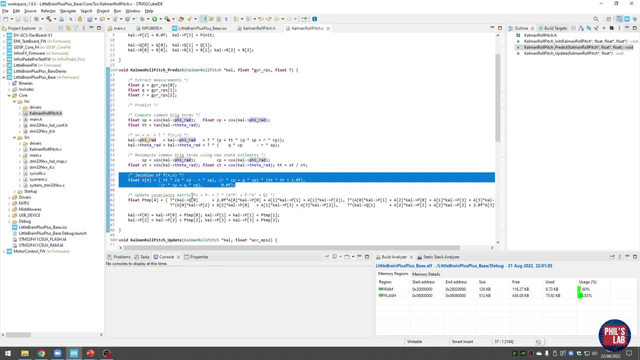 So this will reduce human error, As long as we've, of course, entered the state transition functions correctly, And that's all. I then take over To compute the Jacobian F of XU. Similarly for the next part, To update the covariance matrix. 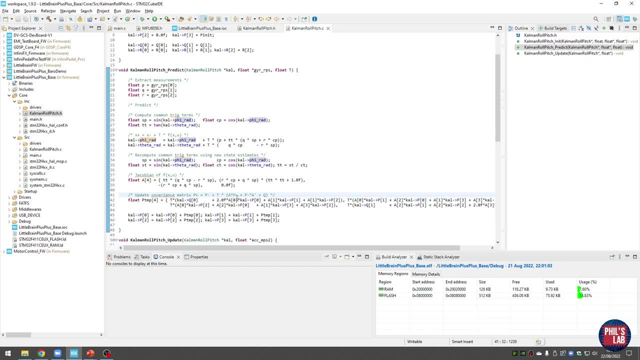 So P is P plus T times A, times P Plus P A. transpose plus Q. Quite a mouthful. I would simply use Octave to do that for me, And that's all I've done, And then I've copied the result over here. 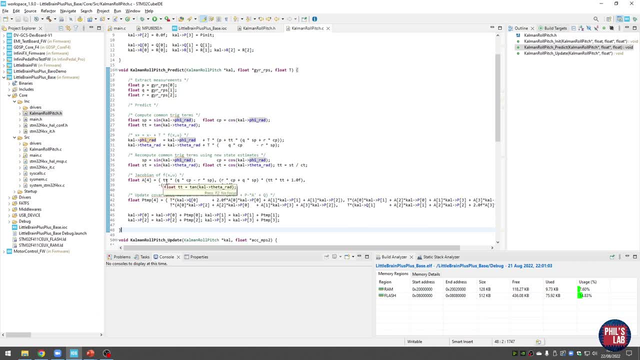 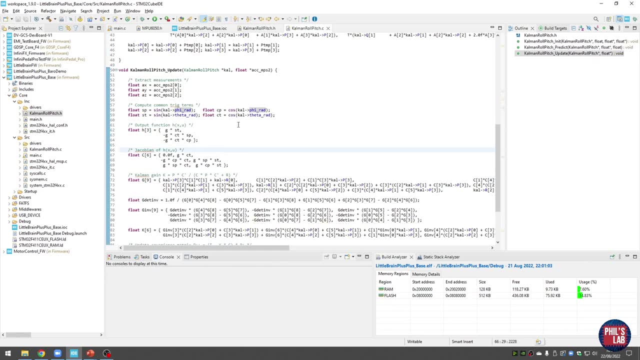 This is all there is to the prediction function. So I'm using the help of the symbolic toolbox and Octave To do this for me And, again, just taking the equations we already looked at, Going over to the update step, I'm doing something extremely similar. 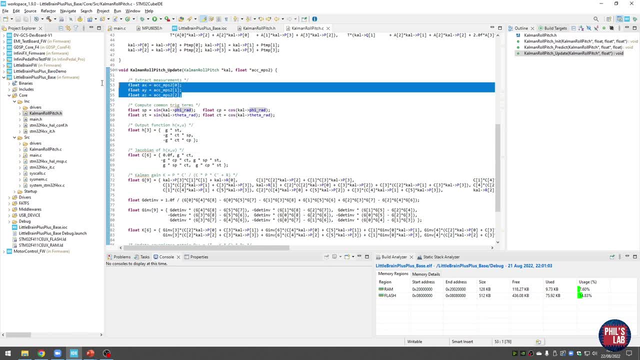 Except this time we have more terms Because we have a matrix inversion. I extract the filtered accelerometer measurements. I compute common trigonometric terms Because we'll be using them again and again. I'm computing the output function from previously Computing the Jacobian again. 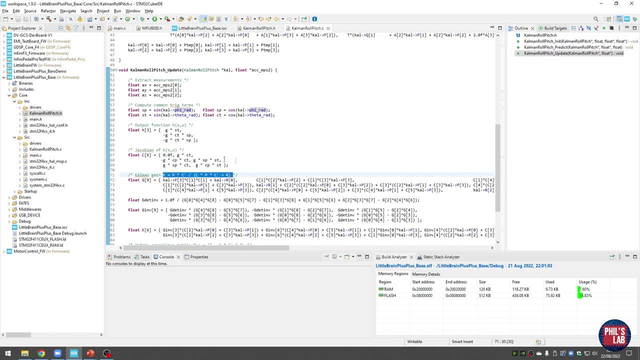 Using the symbolic toolbox And then I'm computing the Kalman gain Including the matrix inversion. So my matrix G Is actually C times P times C, Transpose plus R. Then I'm calculating the inverse of that matrix, Preparing myself for an inversion. 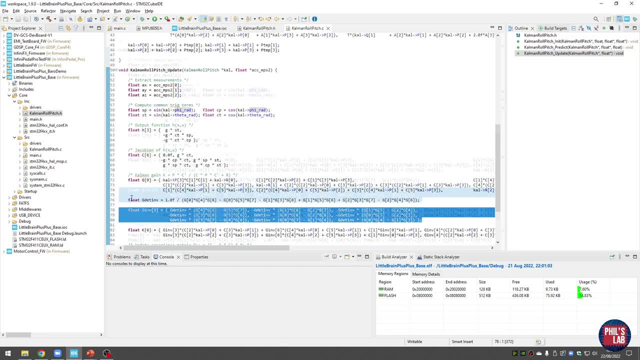 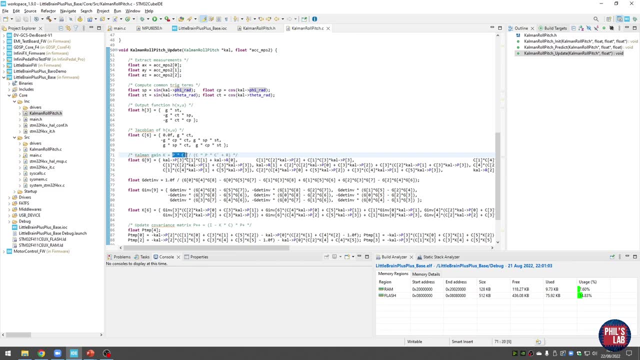 And then calculating the inverse of a 3x3 matrix, This result, This part of the expression here, So 1 over C times P times C transpose, plus R. I'm multiplying by P times C transpose, Which gives me my Kalman gain. 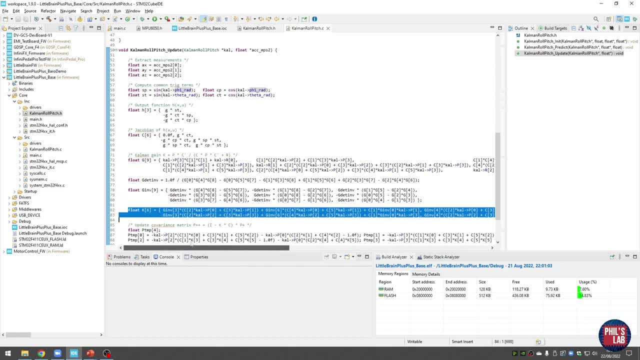 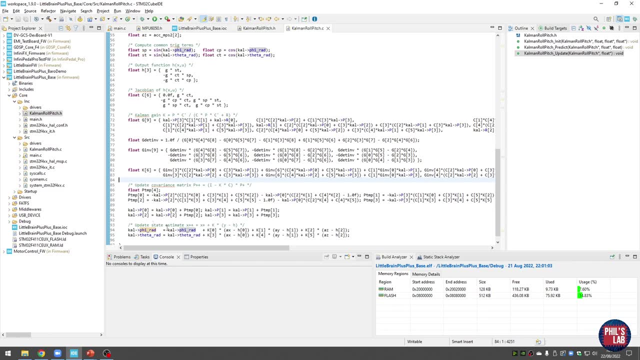 Now, this is quite hefty If I had to do this by hand. And remember, this is only a 3x3 matrix, So this is why I do this with a symbolic toolbox. The next step is then to update the covariance matrix, Again using the formulae. 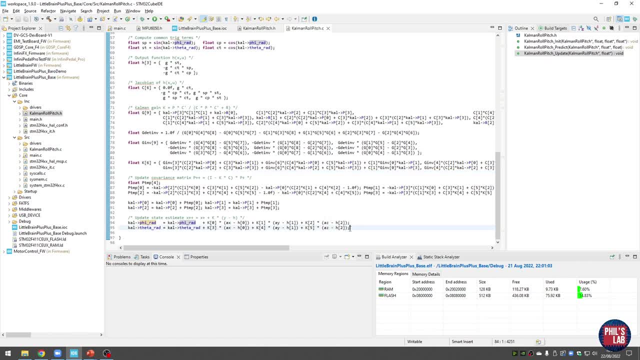 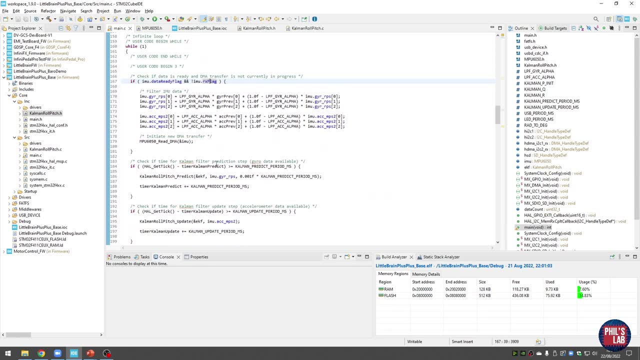 And again using the symbolic toolbox And finally using the Kalman gain And the accelerometer measurements To update my state estimates In main dot C. All I then have to do Is if it's time for my filter prediction step. So gyro data is available. 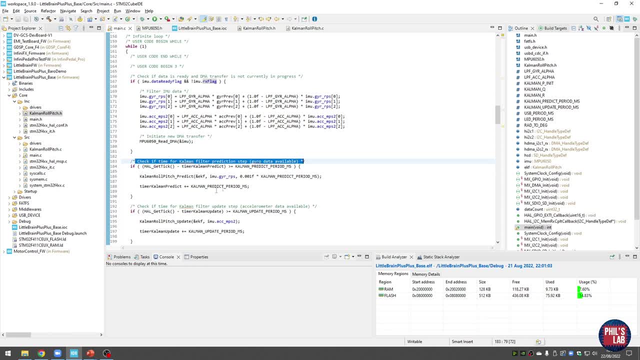 In this case, I'm just running a timer Which runs faster than the update step. So every hundredth of a second I'm running the Kalman predict function With my filtered gyroscope data And my Kalman prediction period as my sample time. 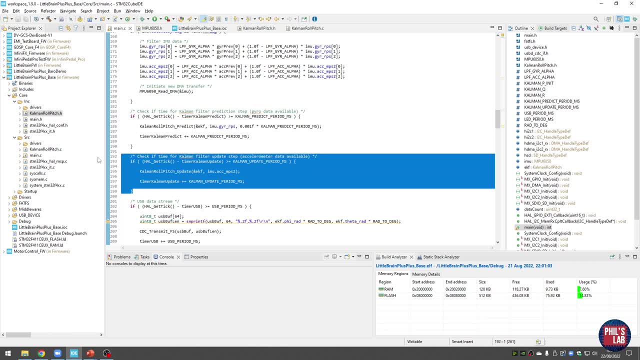 On the other hand, for my update step, Essentially any time accelerometer data is available- I'm again using a timer Which is slower than the gyroscope data, So 10 times per second. I'm simply calling the Kalman update function, Passing in my filtered accelerometer data. 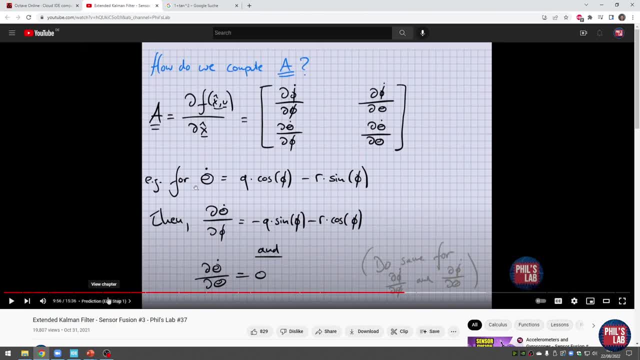 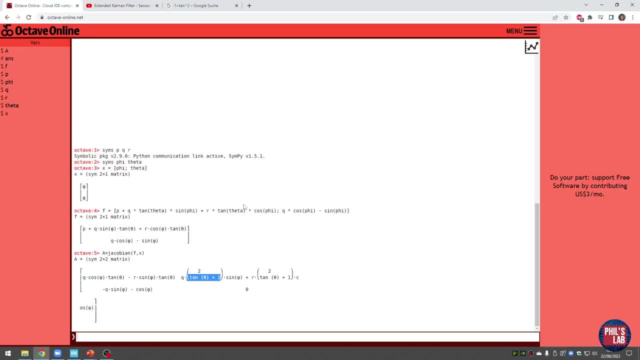 And that's all there is to it. Now, I know that I've glossed over quite a bit of it, And I do recommend going through the previous video To see if you can come up with a C implementation Using these equations In the description box as well. 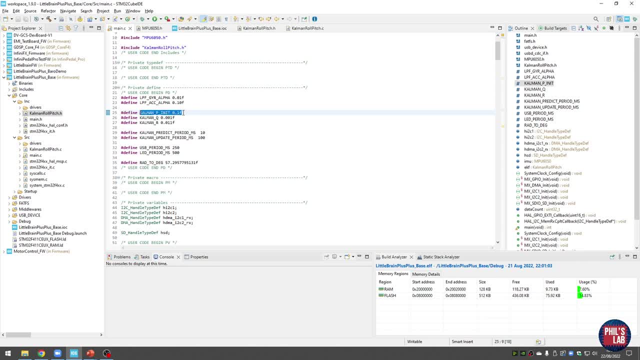 With regards to covariances, I'm simply setting the initial covariance to 0.1.. I'm setting my process noise to 0.001.. And my measurement noise To higher, at 0.01.. Or slightly above. My prediction period is 10 milliseconds. 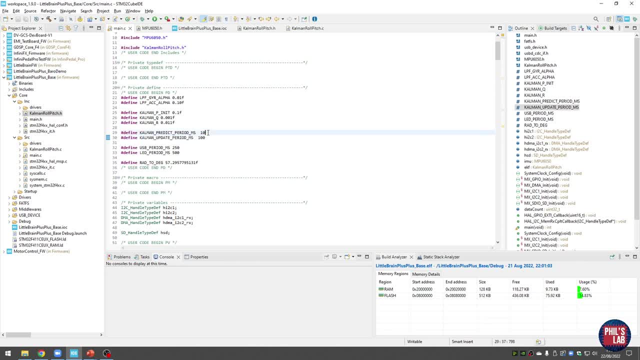 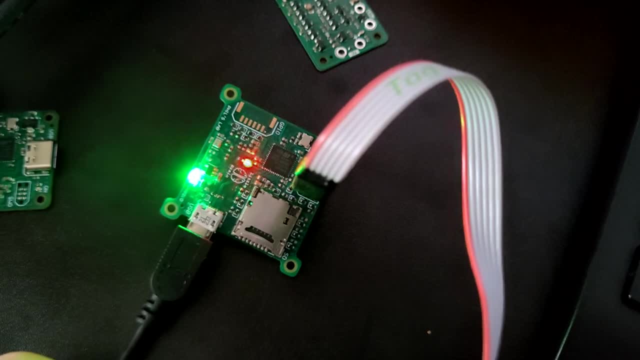 And my update period is 100 milliseconds, And this is pretty much how it would be in most situations. Your prediction is going to run much faster than your update, So let's upload this to the board And check out the results. Now I have the little brain plus plus plugged in. 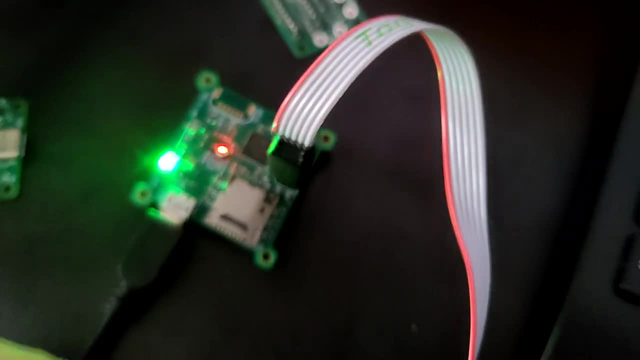 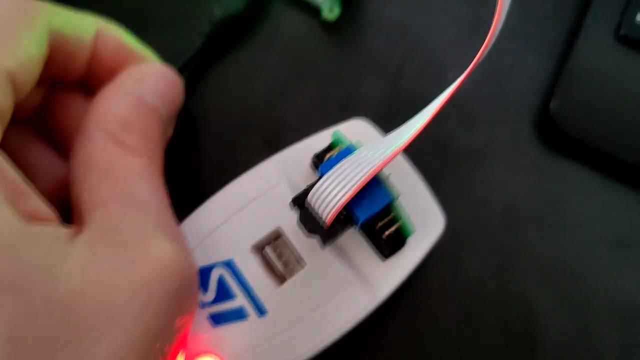 With my USB cable Going to my host PC And I'm also using this tag connect probe, Which is a JTAG or serial wire debug probe Going into my ST-Link V2.. Again via USB to my computer So I can debug and program this device. 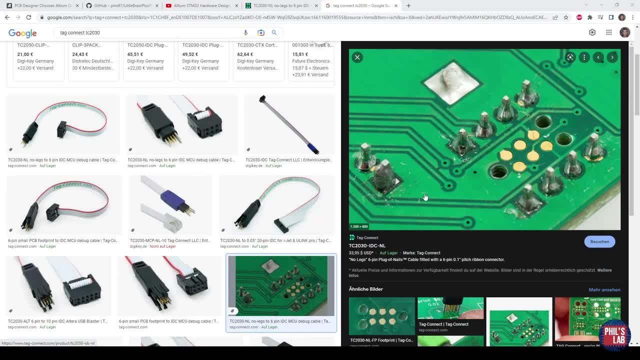 The tag connect probe I'm using to program. this device Is actually pretty cool. So instead of having to use a dedicated header And solder on connectors, We simply have these pads And we have this mechanism That then clips on and plugs in. 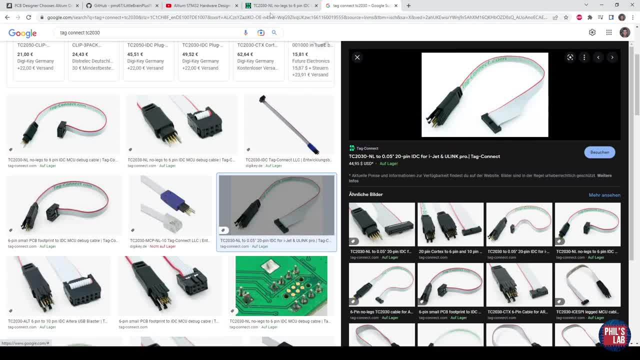 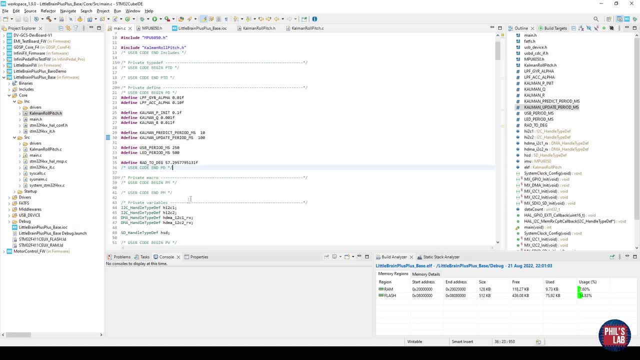 We don't have to solder on connectors, We don't have bomb costs, and so on. The specific one I'm using Is the TC2030. And I'll leave a link to this in the description below. I've uploaded this code to the board. 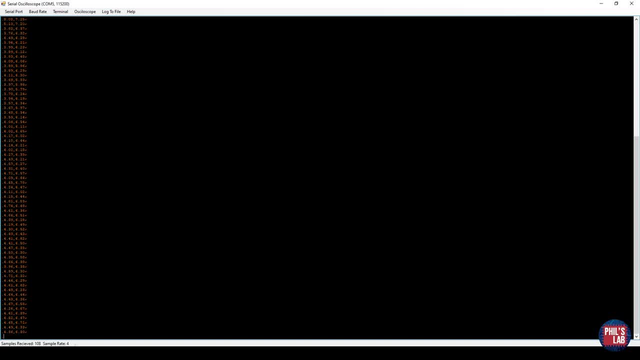 And, as usual, I'll be using this serial oscilloscope To log and plot this data. The sample rate coming out from the USB port Is at 4Hz, So rather slow, But keep in mind that the EKF is actually running much faster. 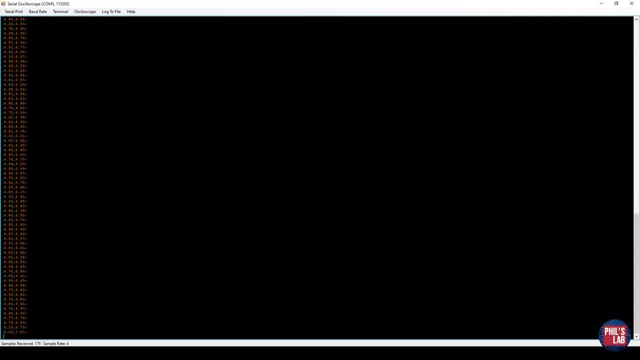 The EKF's prediction step is 100 times per second And the update step is 10 times per second. So now I have the board pretty much flat on the table. We have roll on the left And pitch on the right side. 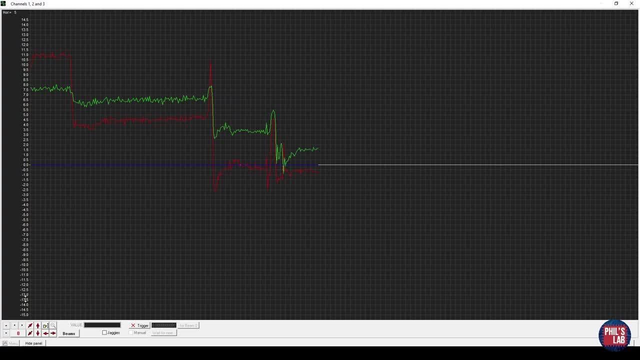 Now keep in mind This is a very crude calibration of the sensors And this calibration and the biases Will drift over time. But now I'm trying to keep the board pretty much flat on the table Roll is the red trace And pitch is the green trace. 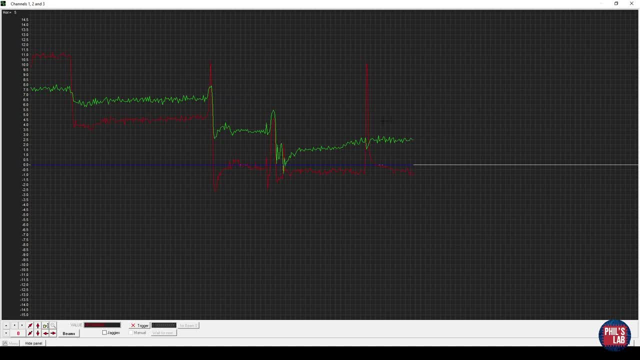 So, nicely enough, It doesn't seem like we're drifting too much, At least over this very short time span. So this is a very crude way of looking at it, And we have close to zero roll and pitch angle, Which is what we expect. 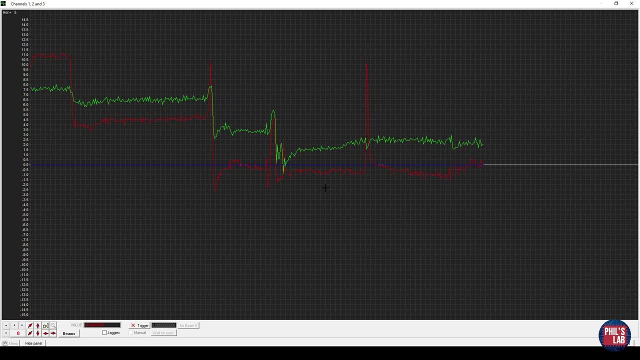 But this board is fairly flat. Of course, my table might be wonky, Which is what we expect to the local earth surface, So this is pretty good to begin with. We have quite a bit of noise on the line, So we might have to change our process. 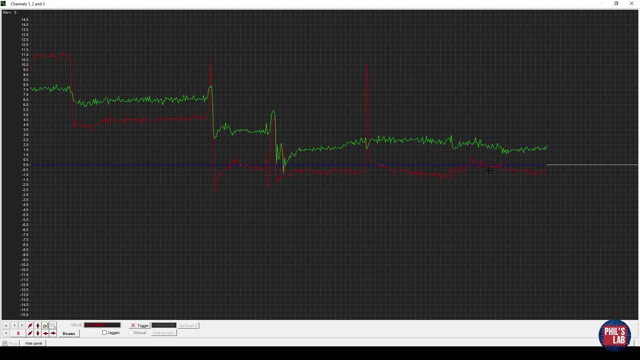 And measurement noise magnitudes, Maybe increase the measurement noise matrix, Or we might have to filter our measurements a bit more. So there's stuff we can play around with In this implementation. So as I try and roll my device, You can see the red curve is changing. 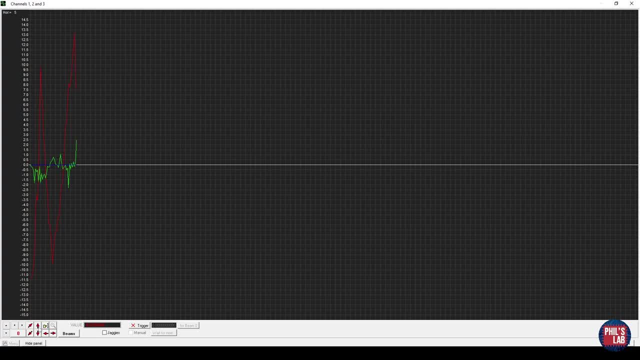 So I roll it to the right And we get a positive roll angle. Roll it to the left, We get a negative one, And the pitch angle is changing as well. Now, this will be due to me Not being able to roll this properly around the axis. 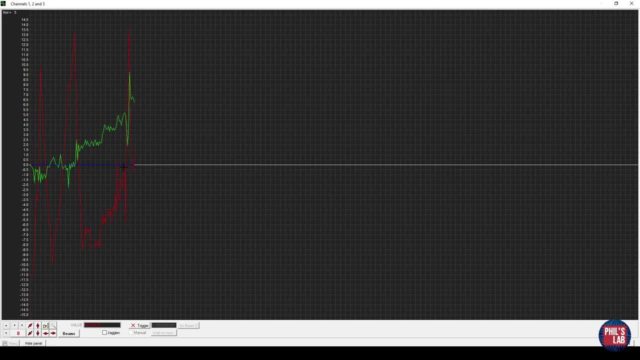 And also inducing some pitch. But there will also be some cross coupling in the sensors Which will distort the EKF algorithm And make it think we're pitching as well. So right now it's very sensitive to movements, So now I can also pitch up. 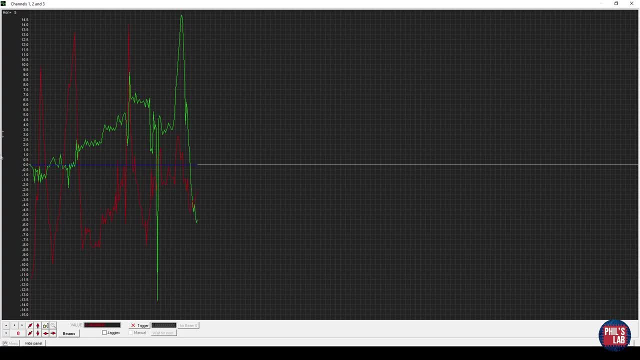 And pitch down. You can also see the roll angle change a tiny bit, But keep in mind the order of magnitude on the left Or the y axis, So I can pitch up and down. I can do both at the same time And you can see the angle goes close to zero again. 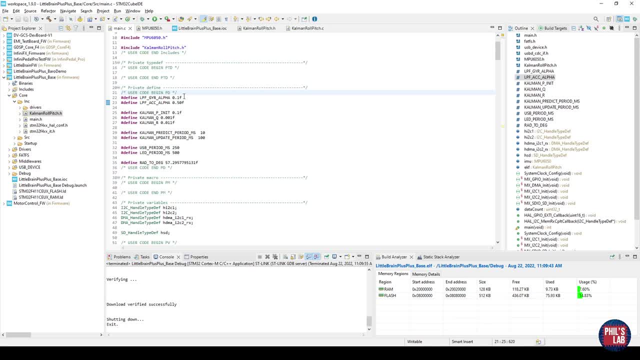 So now I've changed my filter coefficients And increased the order of magnitude. So ten times for the low pass filter gyroscope alpha And I've five times my accelerometer alpha filter value. Going back to the plot, You can see we've definitely smoothed out the trace. 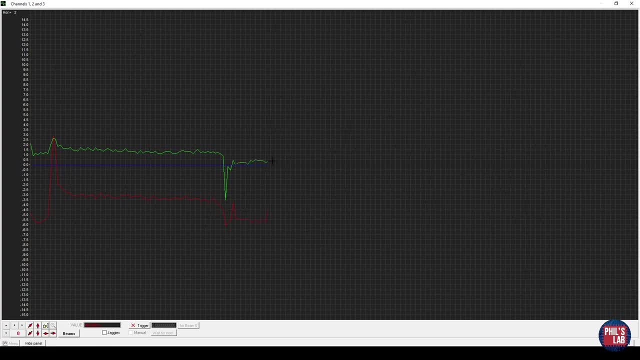 Quite considerably And we're getting a similar response in pitch and roll. So that's an improvement we can make By filtering the accelerometer and gyroscope values Just a bit more. Of course, this will introduce some lag into the system as well. 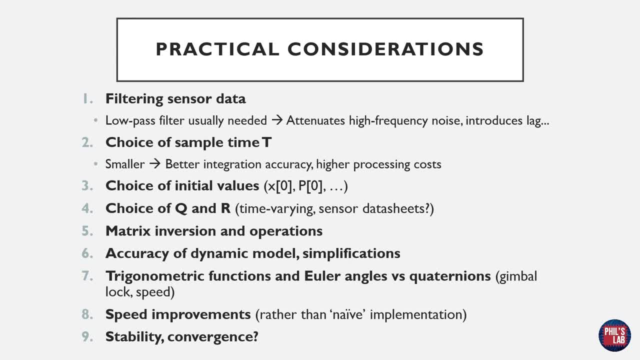 For the sake of time, I've glossed over a lot of the intricate details Of extended kalman filters, Especially when it comes to implementation. There are whole books written on just the implementation part Of extended kalman filters And a video of this length, of course. 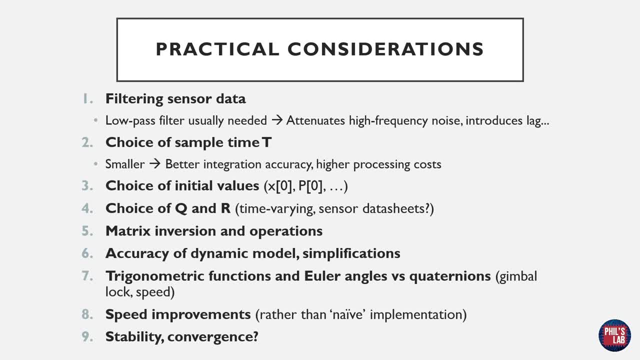 Can only cover a fraction of that. There are some more practical considerations I'd like to leave you with. First of all, the filtering of sensor data. So we've already seen that a low pass filter is usually needed, Attaining its high frequency noise. 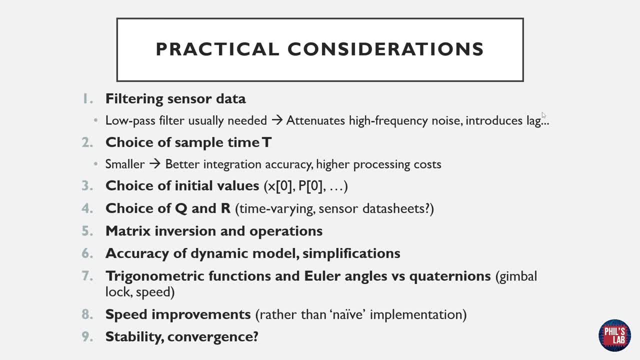 But of course that will introduce some sort of lag Or some sort of delay Which will influence your final measurements And the state estimates. There might also be better filters to use, With a sharper cutoff and so on. The choice of sample time: 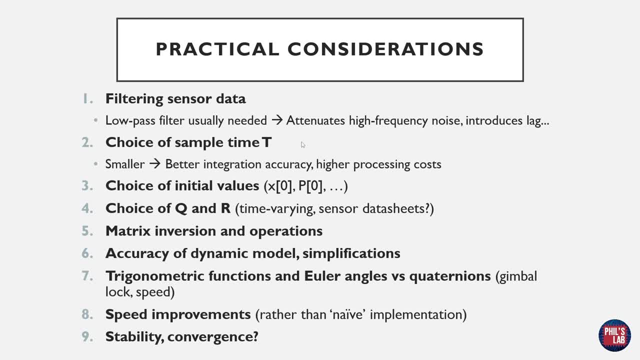 T is also critical. Smaller is usually better, Because that will give us better integration accuracy. On the other hand, you might use a better integration scheme. Running this algorithm at a higher sample rate Will induce higher processing costs. Can the microcontroller even handle that? 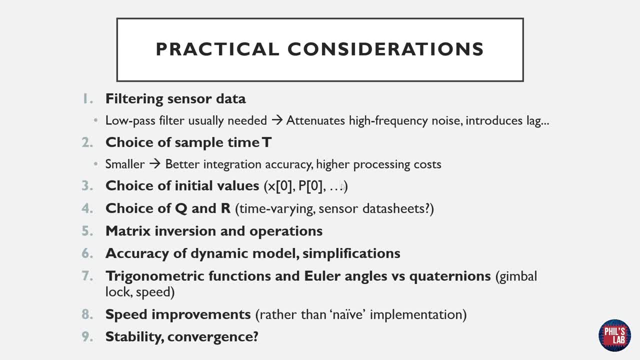 And we might have other tasks running on the microcontroller as well. The choice of initial values for the state estimate And covariance matrix Will also influence how your filter performs, And even if this filter converges The choice of Q and R. 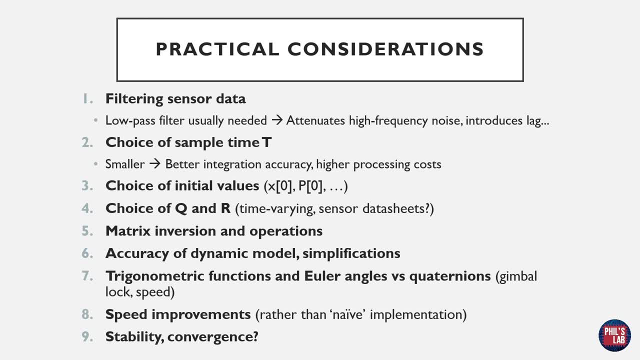 Is probably the most time consuming part Of an EKF implementation: Tuning these properly. You might be time varying. You need to look at sensor data sheets And you need to tune this manually, Based on empirical evidence. Matrix conversions and operations are very costly. 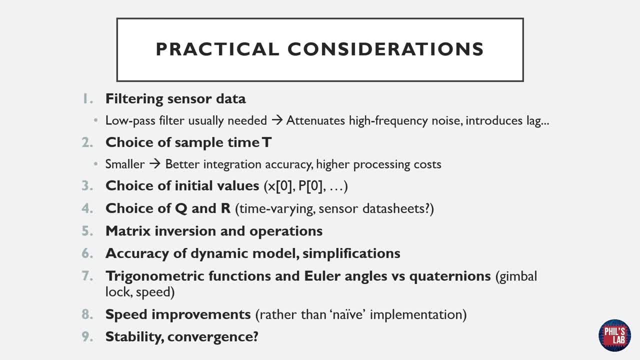 And even though I've shown you a really easy way of doing this By using the symbolic toolbox, Of course this isn't the most efficient way. You might have, often times, sparse matrices And there's algorithms that can exploit the sparseness. 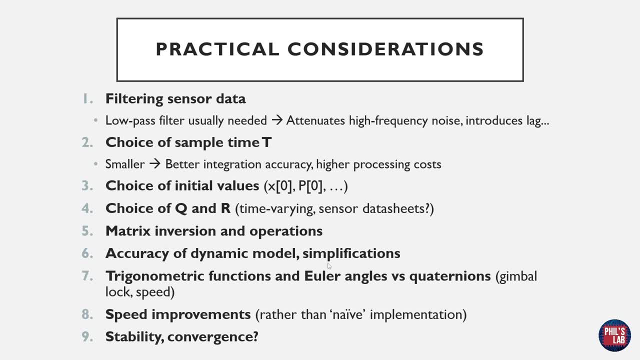 For better and faster matrix operations. We've also used a very simple dynamic model. We've had many simplifications, And a more accurate model Will, of course, improve your state estimates. I've also used trigonometric functions And Euler angles rather than quaternions. 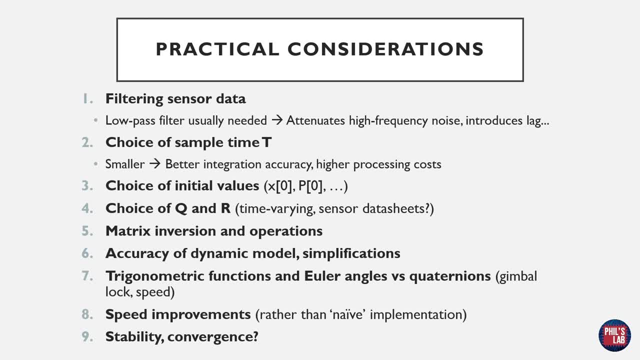 For the sake of simplicity And being able to maybe understand it slightly better Than using quaternions. However, we have problems with gimbal lock, We have problems with speed, Because trigonometric functions are rather expensive to compute, And so on.